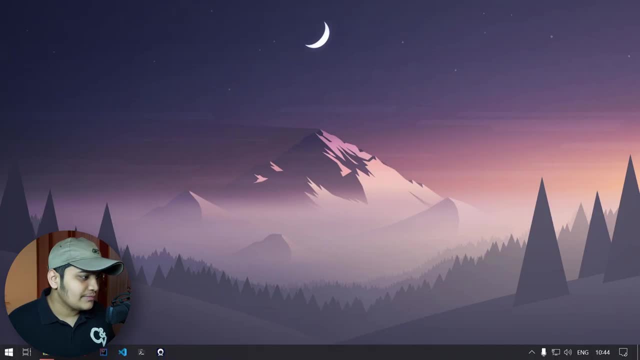 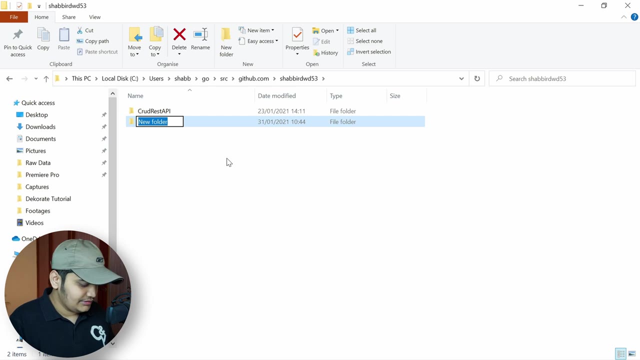 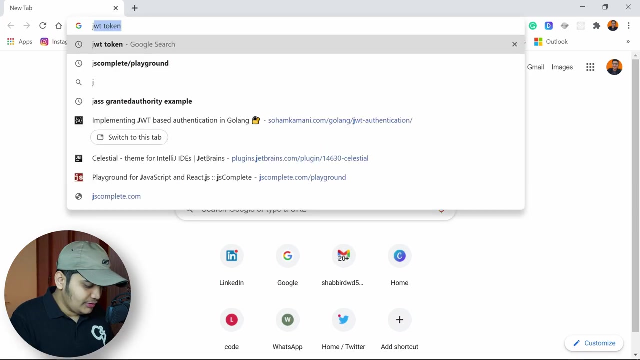 we can work through the JWT tokens. Let's go to the go path over here. Okay, so this is my go path. here I will create my application. Let me just create the application JWT tutorial. I will say okay And let's open in VS code. Now, if you want to know more about JWT, you 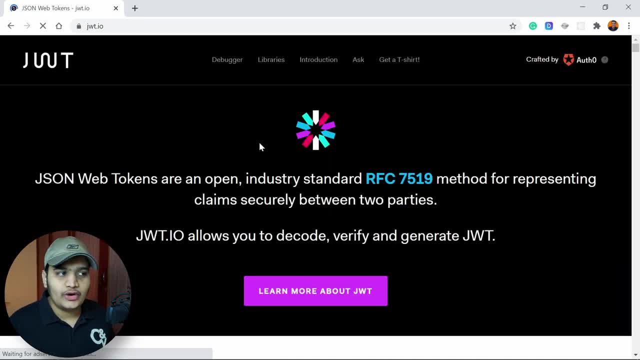 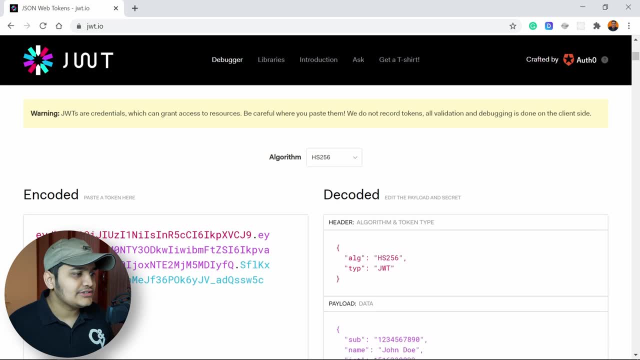 can go to JWT web tokens jwtio website and you can see all the details about the JWT. So yeah, there is also a debugger available over here where you can pass your JWT and you can see the details over here. in the payload itself It will show all the details, your 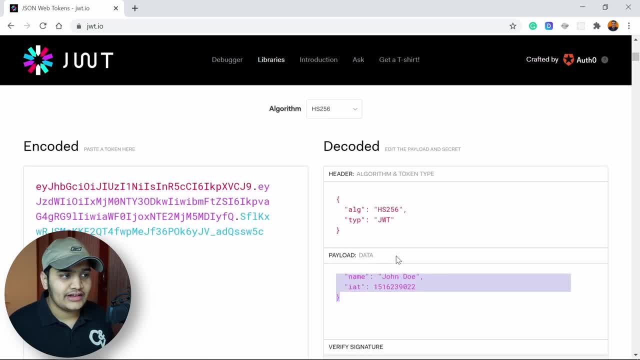 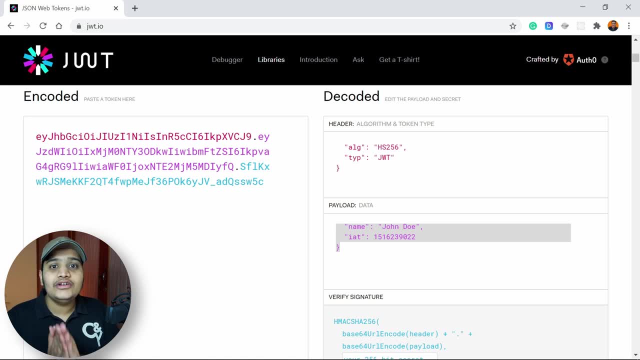 header part, your data part and the signature itself, like what type of algorithm that you have used to create your JWT? what is the payload data of your JWT? it is always advisable to not to store password in your JWT. Okay, because it is visible. It's in public token over here, Okay, so if you want to see any time that, what is your? 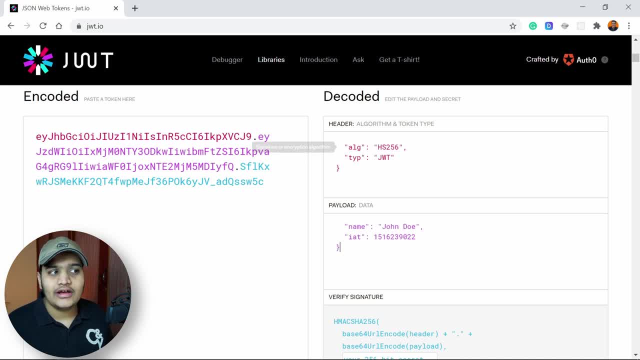 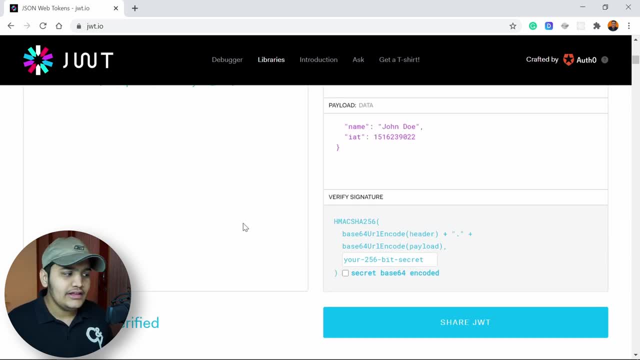 JWT token and what data it is having and what particular algorithm it is using. then you can come here, you can paste your JWT token over here and you will get all those information over here. Now let's go ahead in the go application. Okay, we'll go to VS code And let's create. 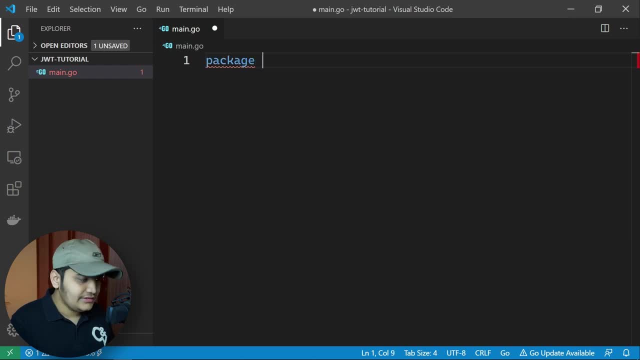 the maingo file over here And we'll say: this is main package and we'll create the main method over here. Now, inside this method, we will define the three handlers over here. So let's define http, dot, handle, func, And here we have to. 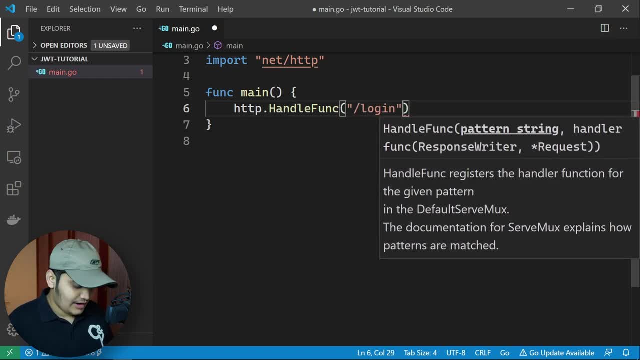 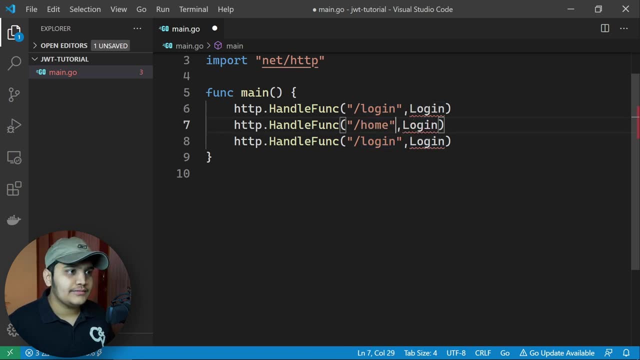 pass the URL pattern will say login And after that we have to pass the handler will say login handler and this will create three handlers. over here will create the home handler. This will be home And here we will create the refresh one. So this handle function is part. 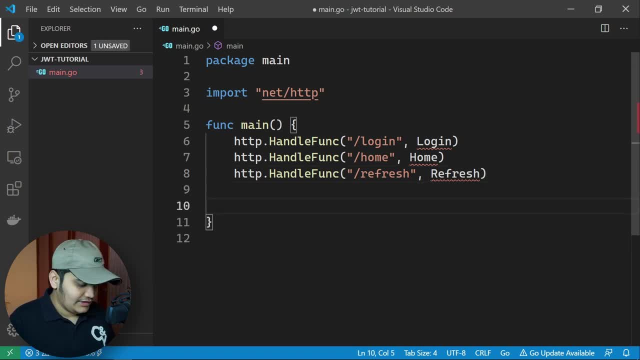 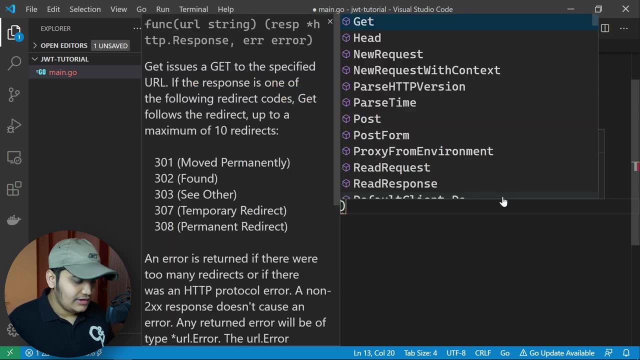 of the net HTTP package. Now we have to start the server, So let's use the log package and print the errors, if it's any, And inside this we'll say http, dot, listen and so, and we'll pass the port information that my application should. 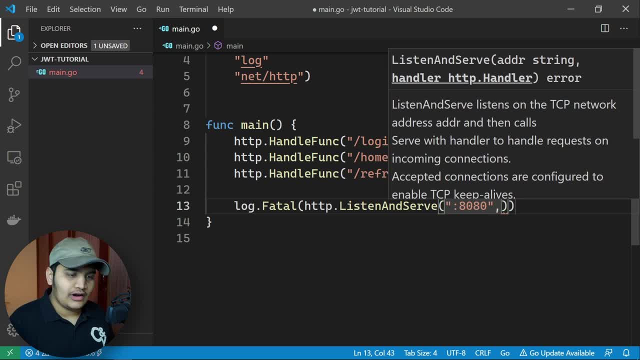 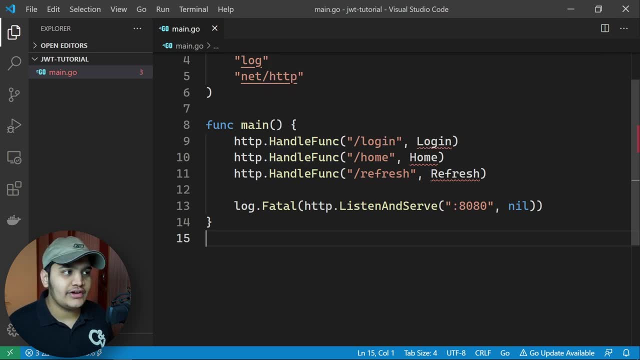 run on port 8080.. And we are not using any router frameworks will pass nil over here. So this is very simple over here, right? We just created the main method and inside this main method we created three handler functions, that is, login, home and refresh, and we'll start. 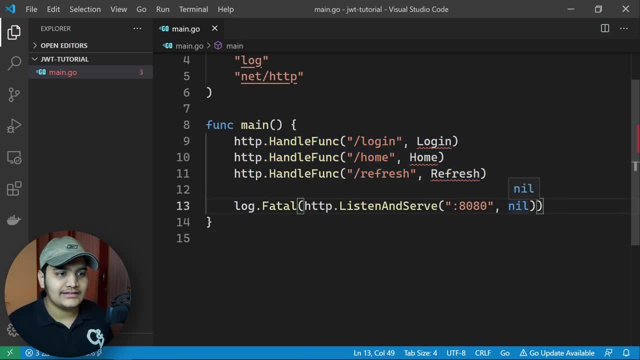 our application on port 8080.. Okay, and we'll pass nil. Now let's create the handler dot go file, and there we will create these three handler functions and we will implement our logic there. So let's create the handlers dot go. 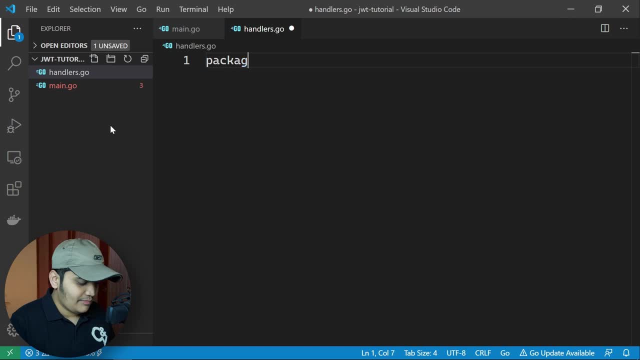 file And this is part of package main. And now let's create these three handler functions and create the handler function. We'll create the home as well And we'll create the refresh as well. This three handler functions are created, which is taking response writer and the reference. 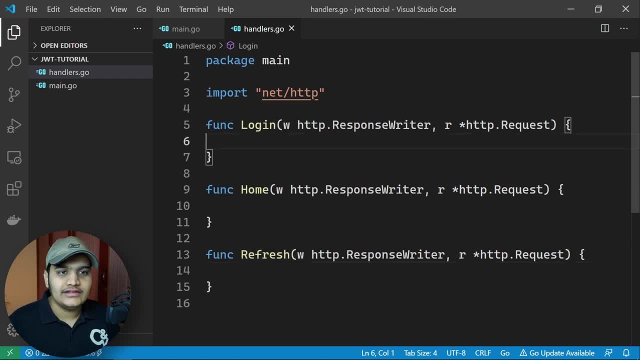 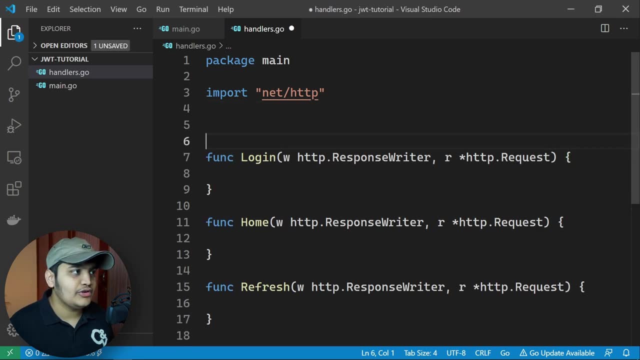 of the request- HTTP request- as the input parameters. Now, in this three particular functions, we will write our code, So let's create a few of the variables we can use over here. Okay, First, we will be using the JWT key over here, So let's create the JWT key. We will create. 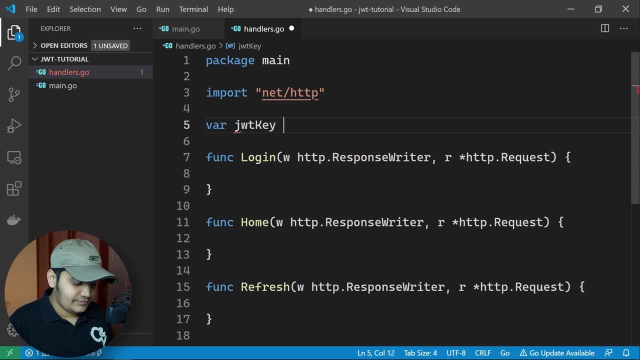 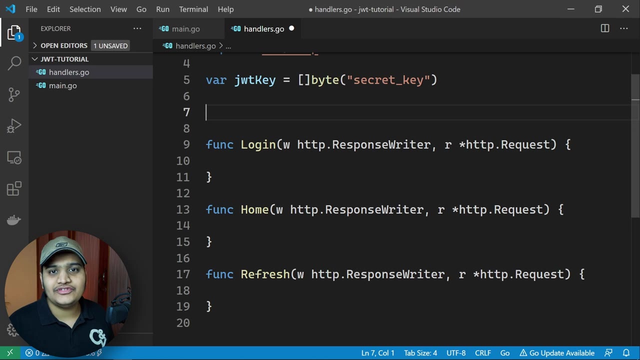 where JWT key equals to it will be byte array And we'll write the byte array And we'll will pass a string as secret key. Okay, this is our JWT secret key that we will use in our JWT token to sign our JWT token. Okay, now let's create one map of a user which will: 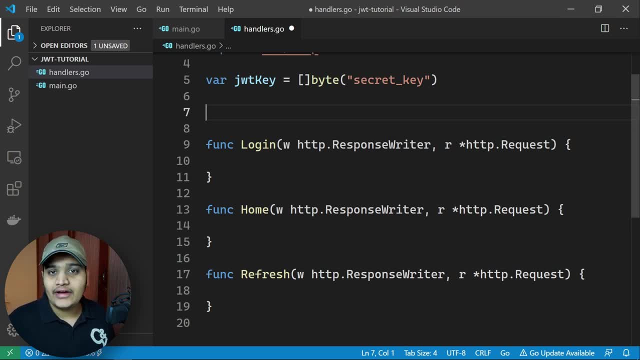 contain username and password. Okay, because we are not connecting to database. generally will be connecting to database and fetch the username and password, But here I'm just creating a map over here. for the sake of simplicity and time, I'll create a map having a couple. 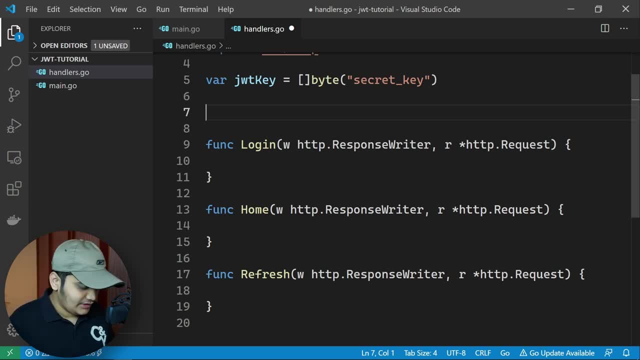 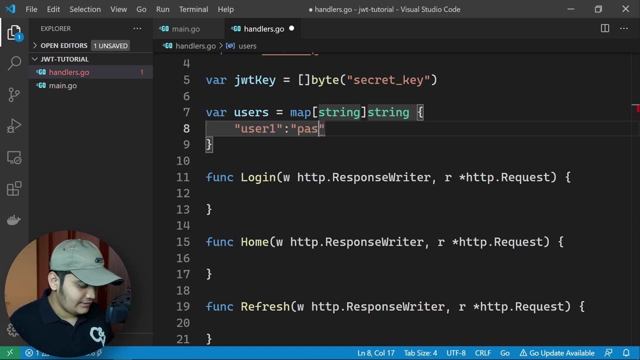 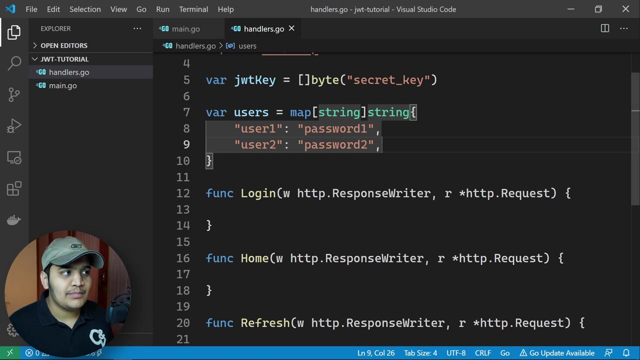 of users and we'll pass username and password over there. So let me just create the map. variable users equals to map of string and string which will contain, suppose, user one and key as password. one will copy paste this information, will add user two and password two. So this is just a simple map that we have created which is storing two users with 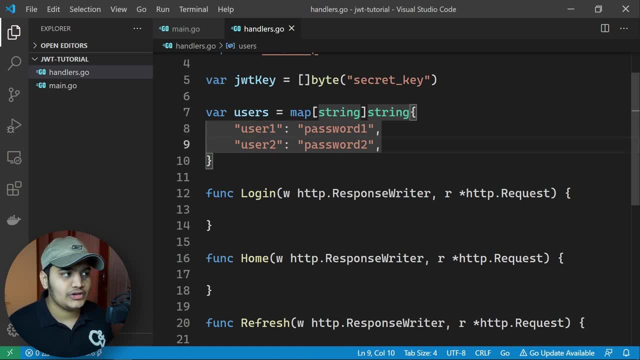 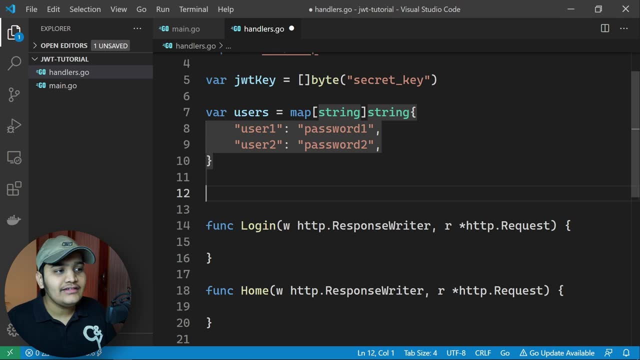 username, user one and password is password one and user two and password two. Now let's create one struct called credentials So we can pass the data as a username and password from the API's and we can use over here. So let's create the structure over here. we'll say type credentials as struct and say: 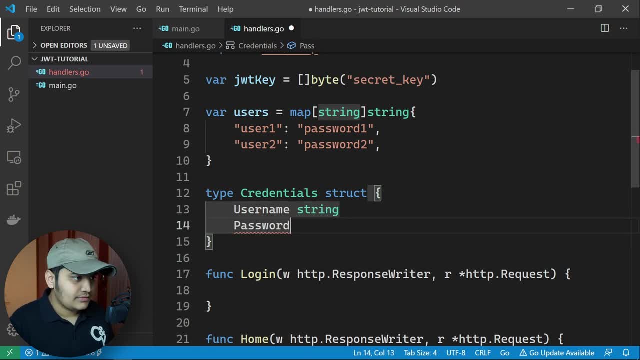 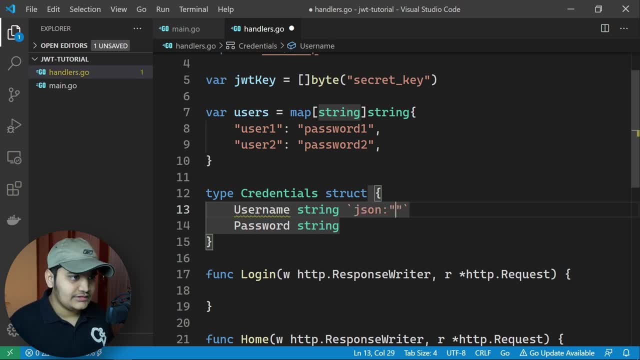 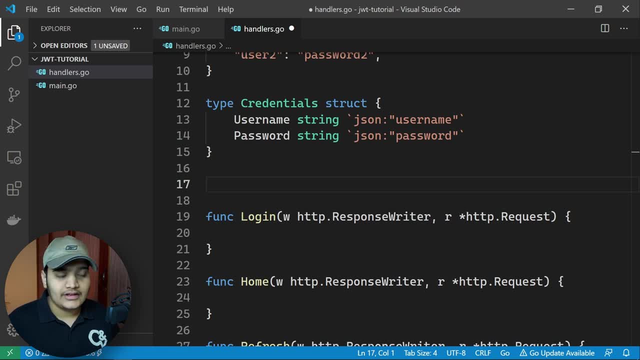 have created. Now let's create one more struct that is called claims, so that claims will be using to create a payload for our JWT. inside that payload we will pass our username and when that particular token is expiring. Okay, so let's create that particular claims. over here We'll say: type: claims of struct. 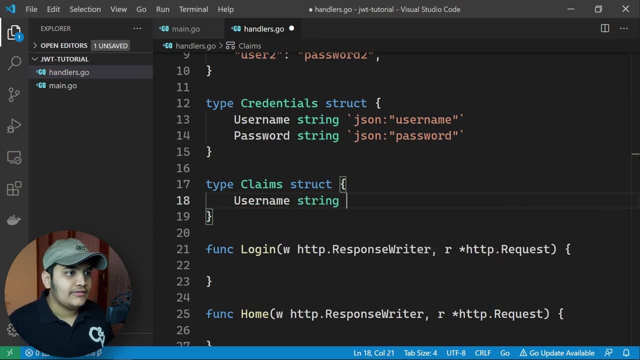 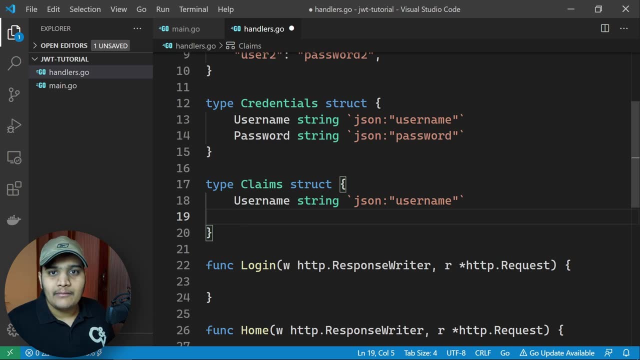 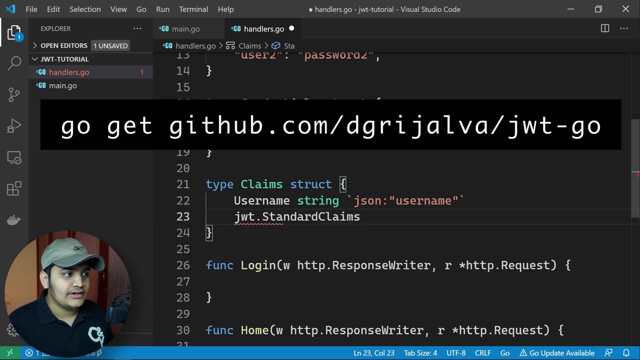 and we will say username string and we will pass this Jason as well, This Jason implementation over here. Now we will embed one standard claim struct over here from the JWT library- JWT dot standard claims over here. So with this we will get the extra information like: 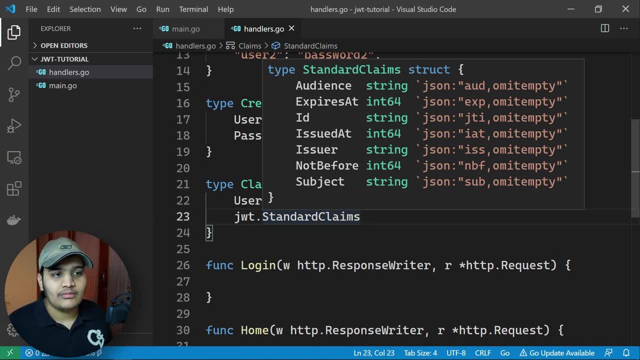 like audience expires it. ID issue at issuer not before subject. So these are the extra particular fields that we can get from the standard claims. We will be using the expired at attribute variable from this particular standard claims for now, but you can use all this as well. 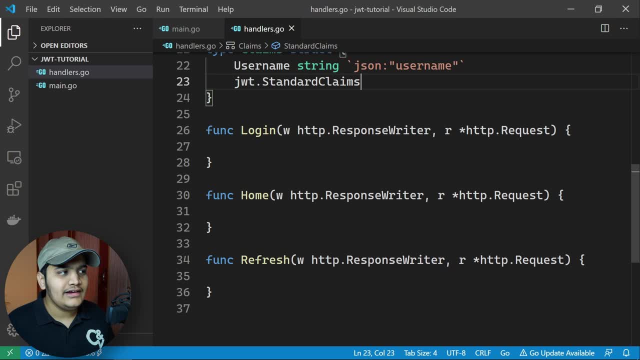 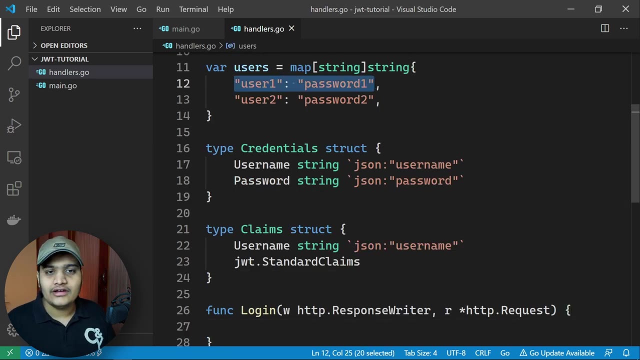 So this is a claim struct that we have created. Now let's go ahead and use the login method and inside this login method, let's implement our logic when the username and password that we are getting from the body of the request, if it's matching with the credentials of the particular map that we have stored over. 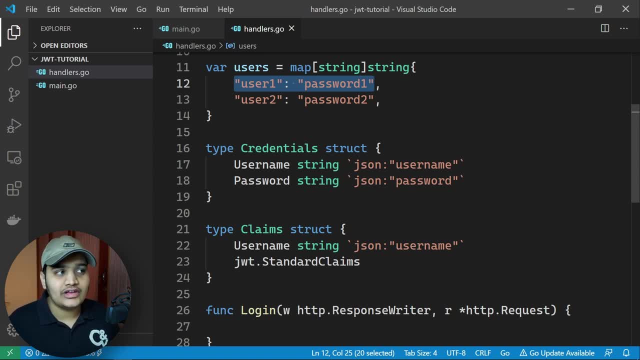 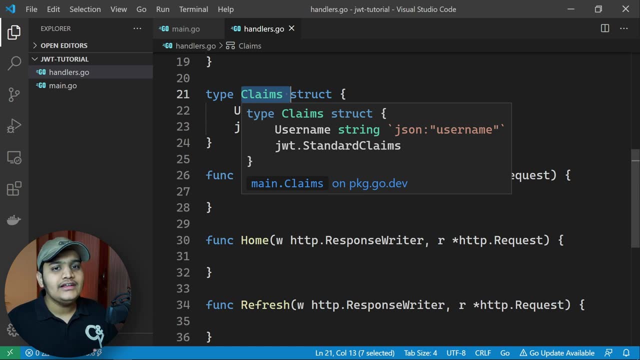 here, or either you can use the database. also, if the credentials and username are correct, then create a claim object for it. Then, after creating the claim object, create the JWT token from it and store the data into cookies and pass the request back. 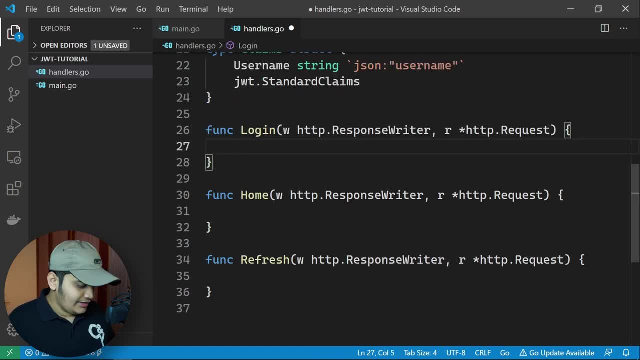 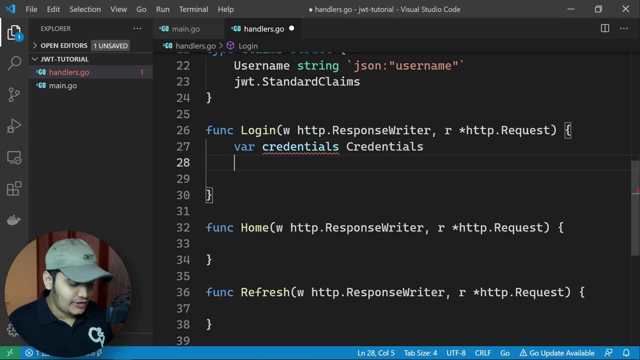 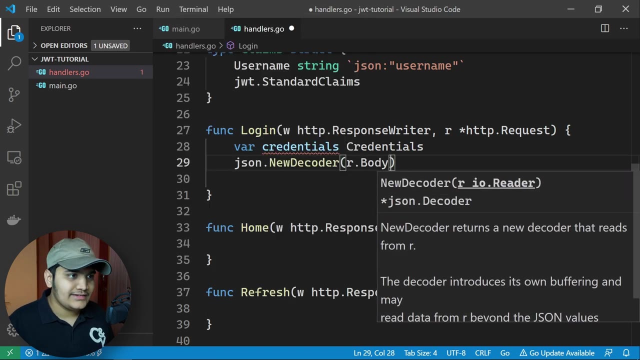 So let's implement that particular logic over here. So here we'll create the object of credentials- credentials of type credentials- and we will take the data from the JSON. So we'll use JSONnewDecoder. here we'll pass the body of the requestdecode to reference. 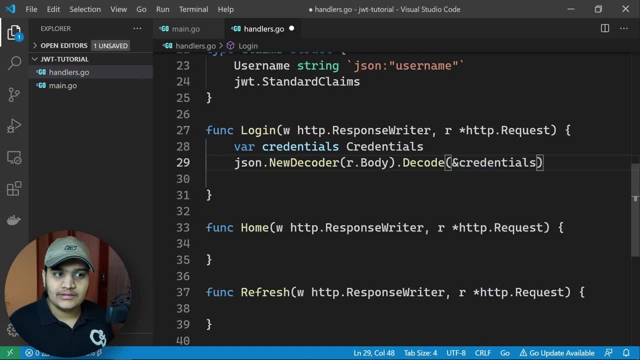 of credentials. So this is a simple thing that we have done over here in the earlier video also, when we created the Go API and mux, we have used this particular syntax over here. You can check that out as well if you are not aware of how to create the REST APIs in. 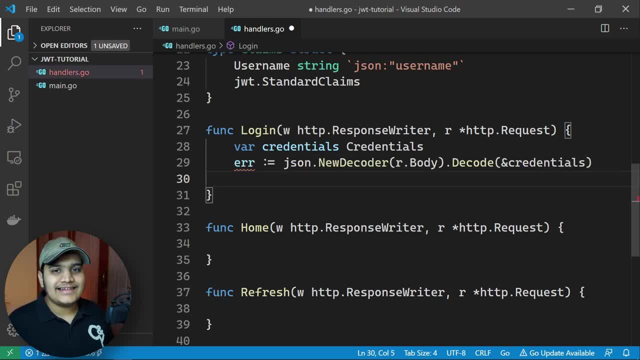 Golang And we will see if there is any error over here And here let's handle the errors. if there is any error while getting the data from the body itself, then we can throw the exception. So we'll just check if error not equals to nil. 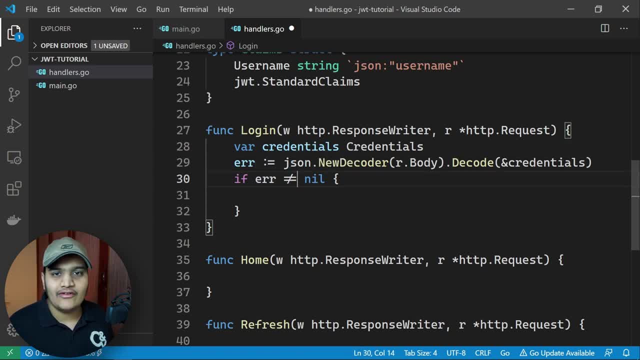 So don't get confused with this particular syntax. This is just not equal to. I have enabled the ligatures in my VS code, So that's why you are seeing this way. Okay, But generally it is not equal to itself. Now, if you are getting any error over here to decode the body, then we will just throw. 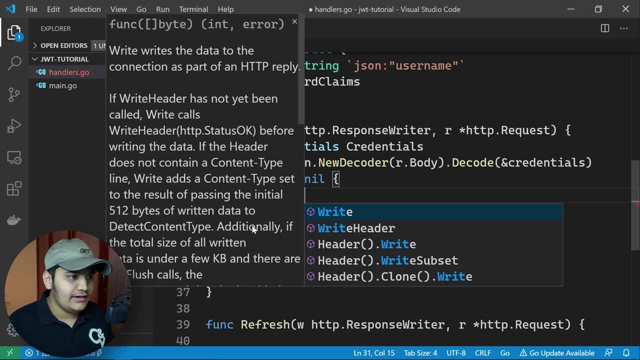 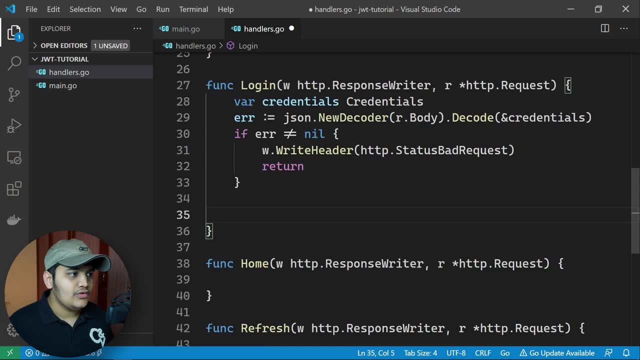 the error back to the client WDDWriteHeader. Okay, And here we'll say status: bad request and we'll return. So we've handled the error over here. Now, if there is no error, then we should get the data in the credentials object over here. 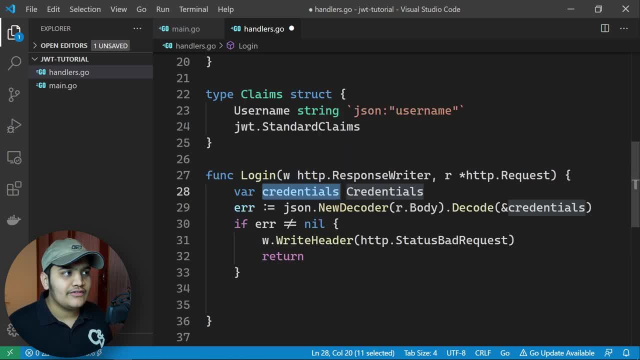 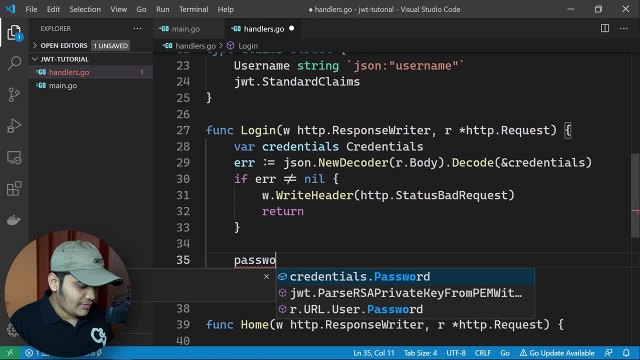 Okay, Struct over here. Now let's match the data of it with the data that we have in our users map over here. So let me store the data of password here. I'll say this is expected password, Okay. Expected password, Okay. 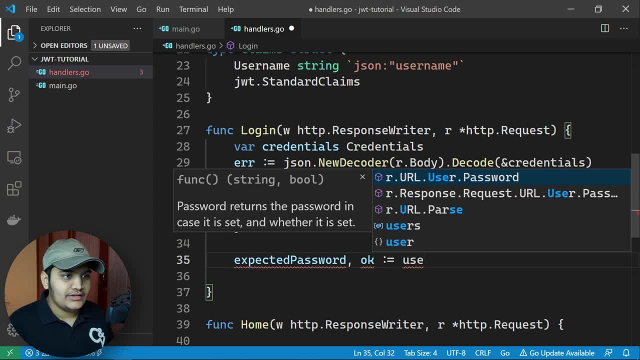 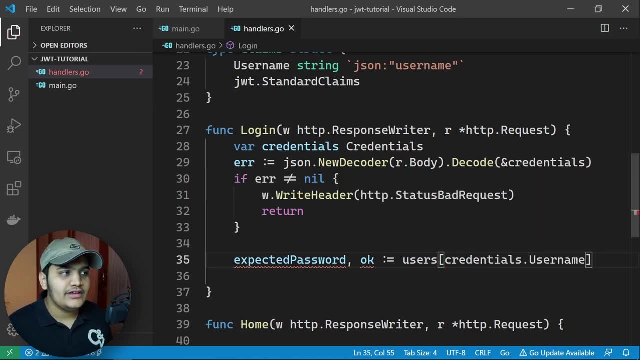 Equals to get the data from the users and here we'll pass credentialsusername. So whatever username we are getting in the credentials object over here with that username we are getting the data from the users map and we are storing in the expected password and okay, variable. 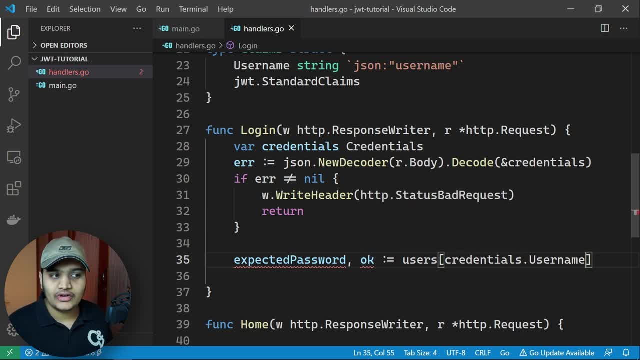 So from this map we will get to know, okay, if the data is available with this particular username. if so, then what is the expected password. So we'll match the username and password both from this particular syntax. Now let's do the if condition. 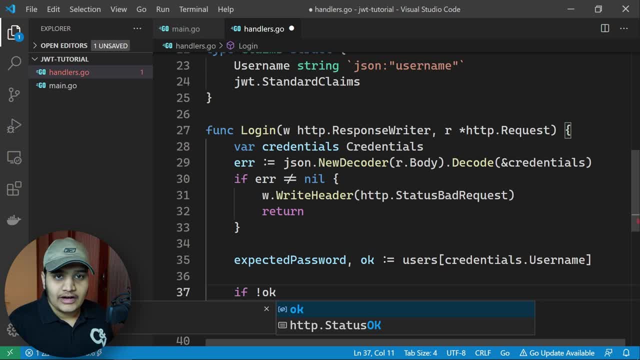 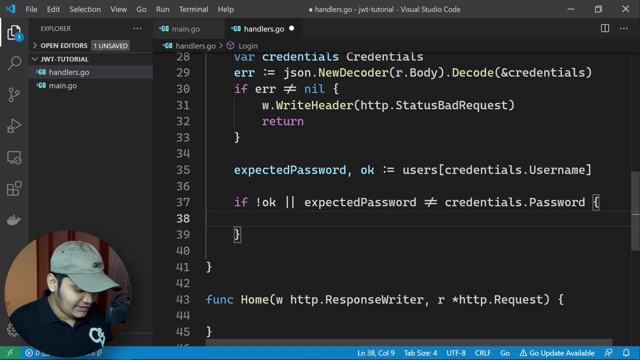 Okay. If not, okay, if the password is not stored or expected password is not equals to credentialspassword, then this request is not authorized. So we'll just say wtwriteheader- httpstatus unauthorized and we'll say return. So we just check the simple thing over here if the password is correct or not. 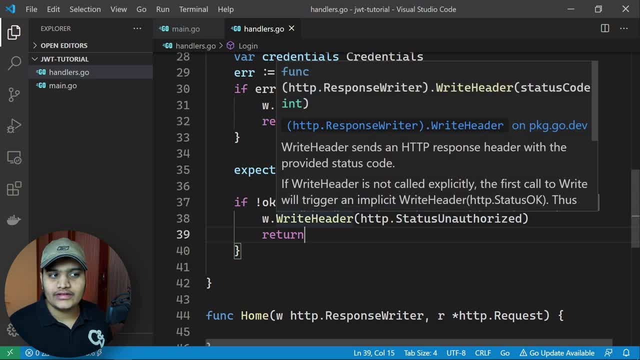 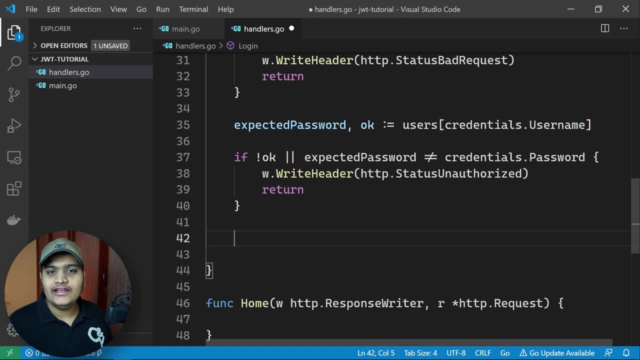 Okay, If the passwords are not correct, Then we are just throwing the error back, that this particular request is not authorized. If the request is authorized, then what we'll do? we'll create the object of a claims and then we have to sign that particular token. 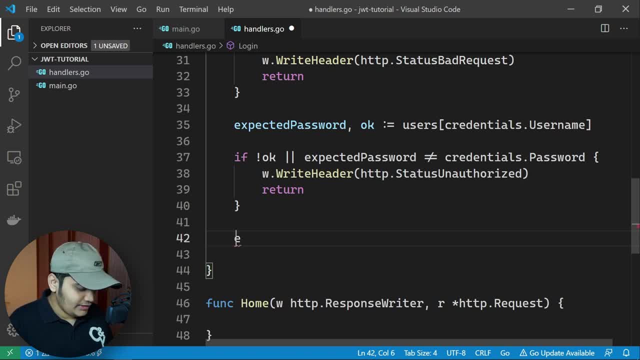 So for that, let's create one expiration time over here. So we'll just say expiration time equals to. we'll use time dot now and inside this we'll add five minutes. Add five minutes. Okay, Time dot minute into five. So what we're doing is we are creating the time over here plus five minutes current. 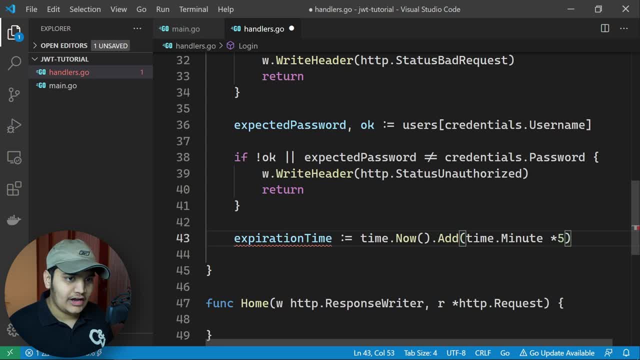 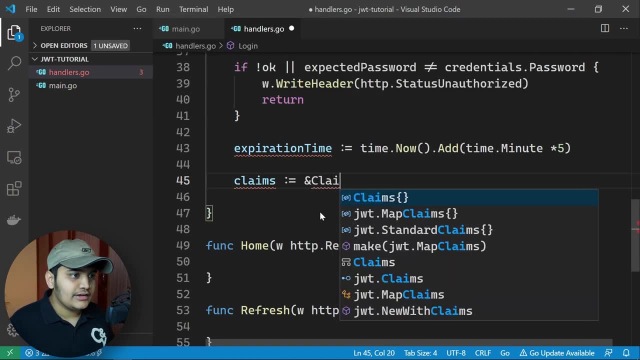 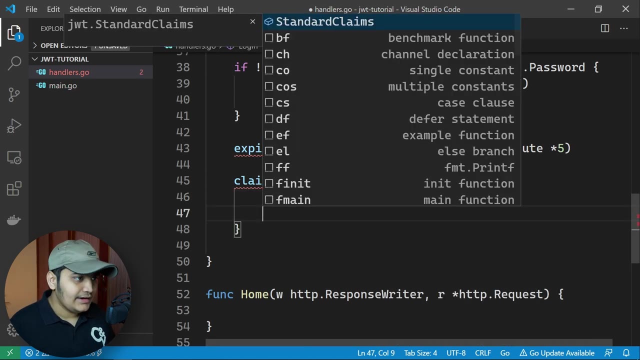 time plus five minutes, So this will be the expiration time of our token. Now let's create the claim over here. So we'll say claims equals to the reference of claims And inside this claim we'll pass username equals to credentials, dot, username and standard. 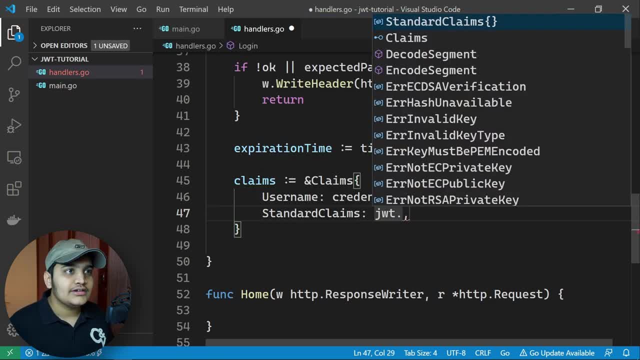 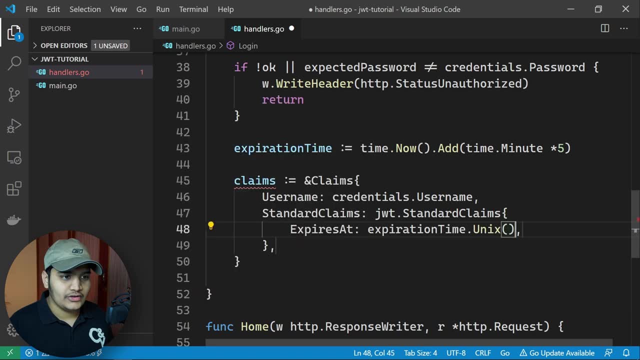 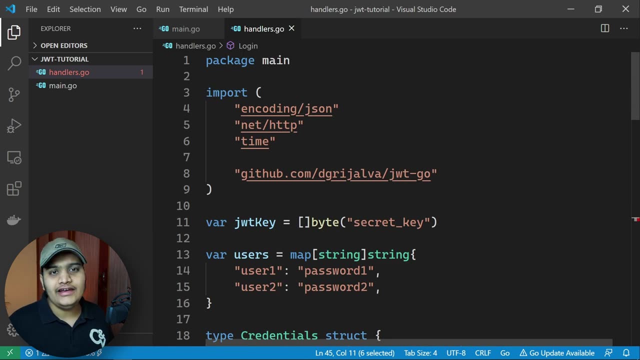 claims equals to JW, JWT, dot standard claims and inside this, standard claims will pass expired at expiration time. dot unix: This particular claims is created. Now we have to use this claims object plus the JWT key that we have defined over here and to create the token out of it. 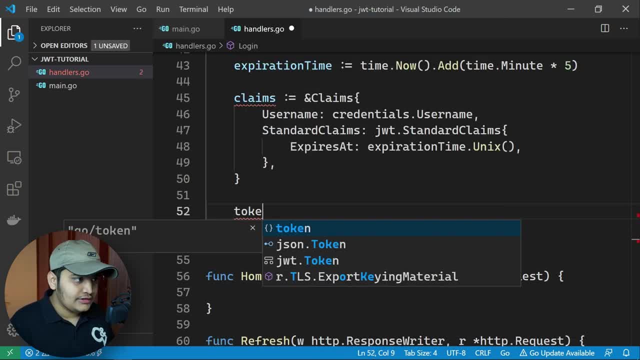 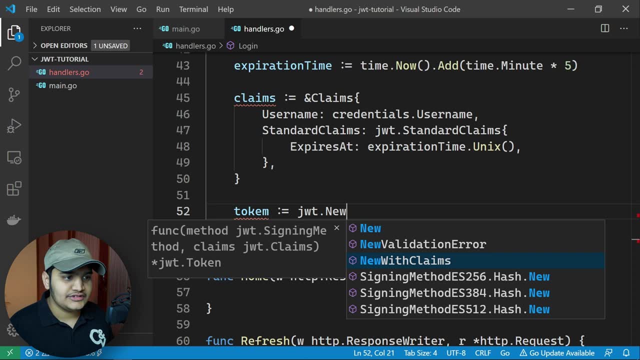 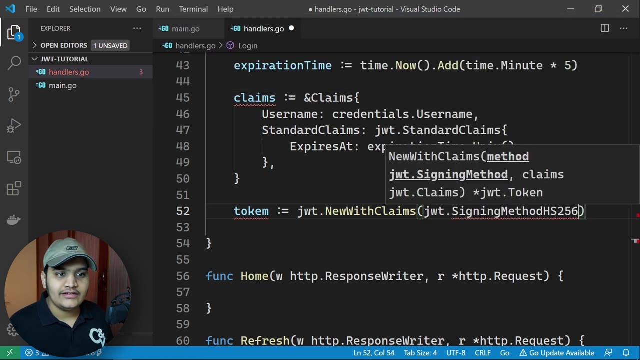 So let's create the token from here. So we'll create token equals to JWT dot- new with claim. and yeah, we need to provide the signing method. So we'll provide the JWT dot will provide the HS256 signing method, and then we have to. 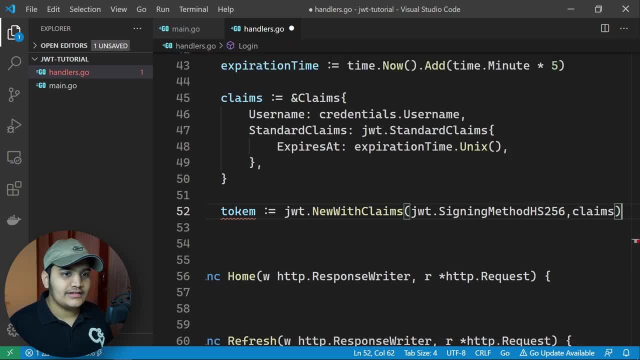 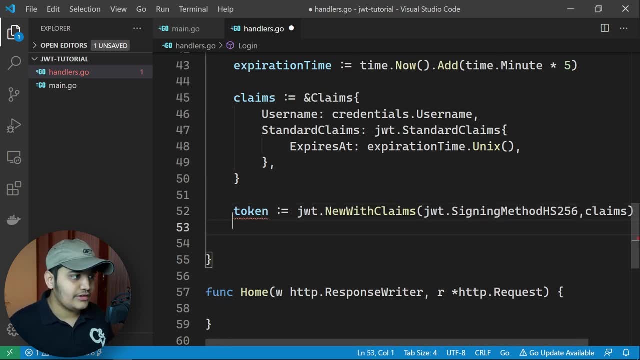 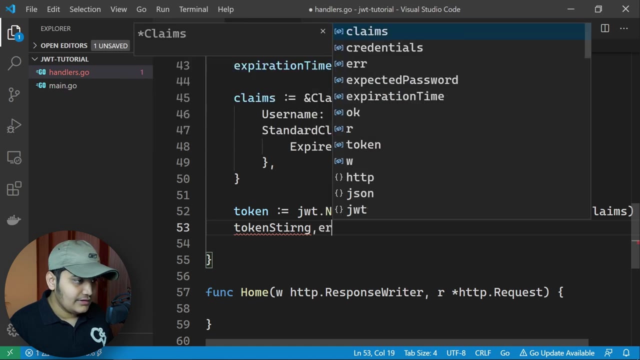 pass the claims over here. Okay, this is simple over here that we are creating the claims over here. Now let me just do token over here and now from this token we will get the token string. So we'll say token string and error equals to token dot sign string. 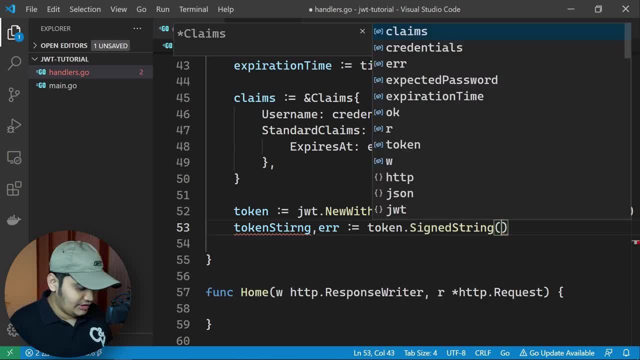 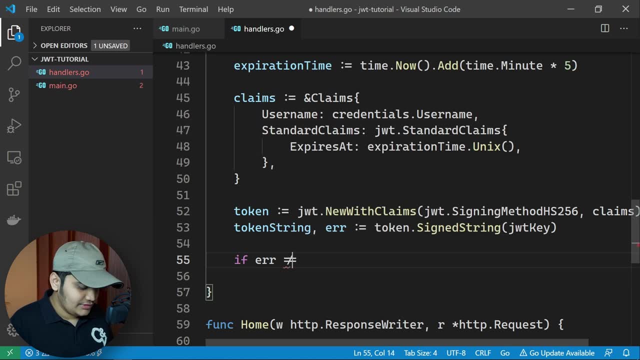 And yeah, And yeah, we have to pass the JWT key spelling mistake. Okay, Now if there is any error over here, if error not equals to nil, we'll say internal server error. w dot write header say internal server error and we'll say return if there is no. 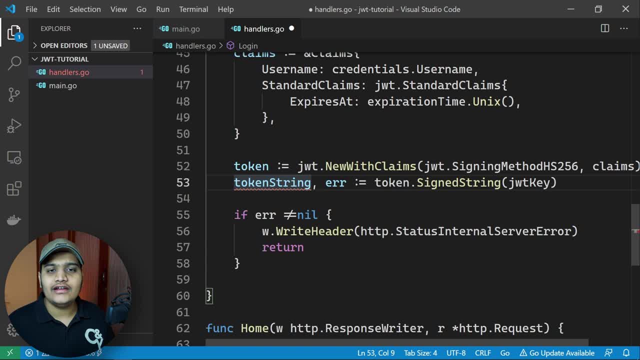 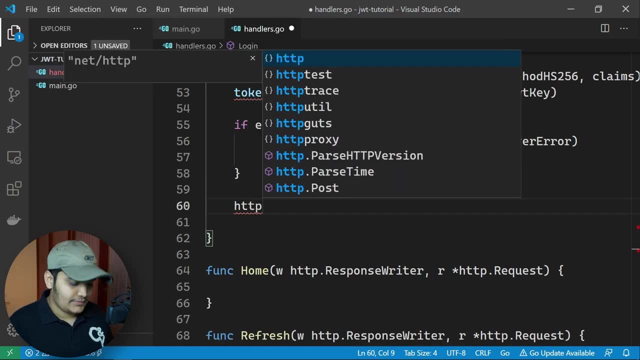 error over here. That means we got our token string over here and we are ready to set those particular things in our cookies. So let's set the cookies over here, Say http dot set cookies, and yeah, we need to pass the writer object and then the reference. 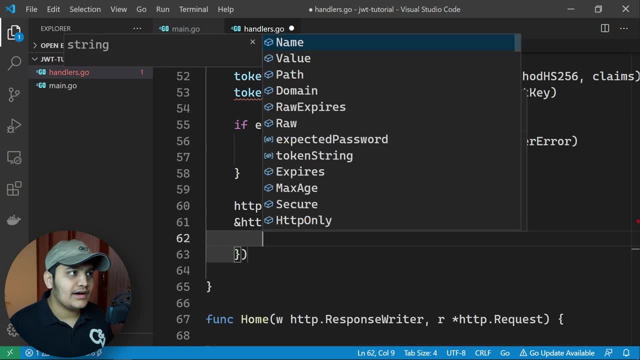 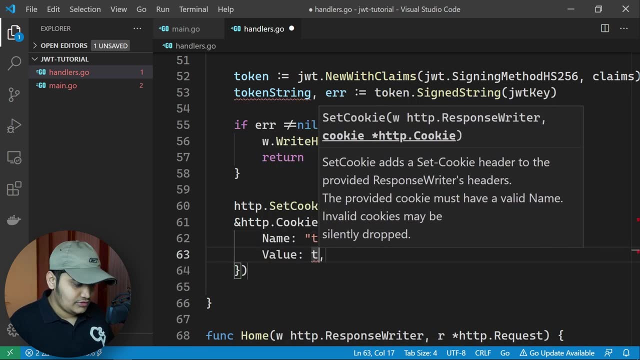 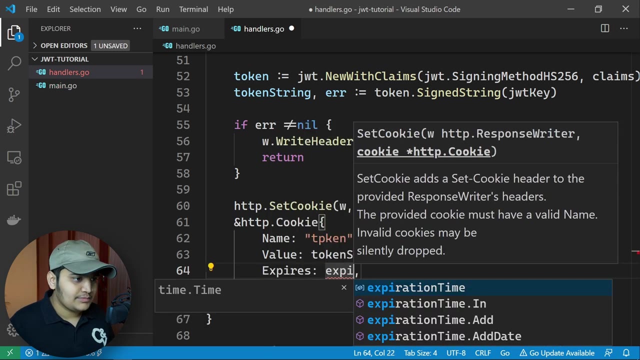 of the http dot cookie and inside this cookie we will pass: name equals to token, then value equals to token string and expires at expiration time. Cool. So this is simple. We have to add the cookies over here with the name of the cookie as token and the token. 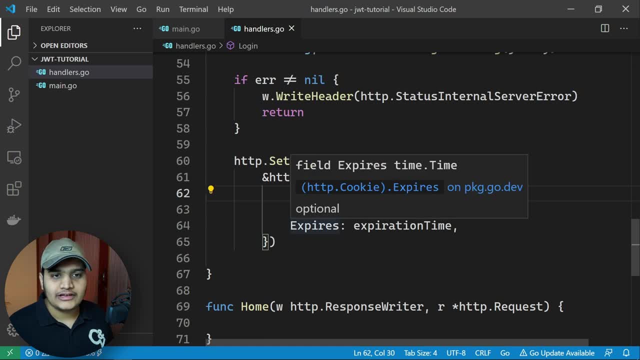 string as the value and expiration time as the expiration time of the cookie itself. So all these values- cookie values- will be stored to our cookie, into our browser or whatever client that you are using. Okay, So this was very simple over here, guys. 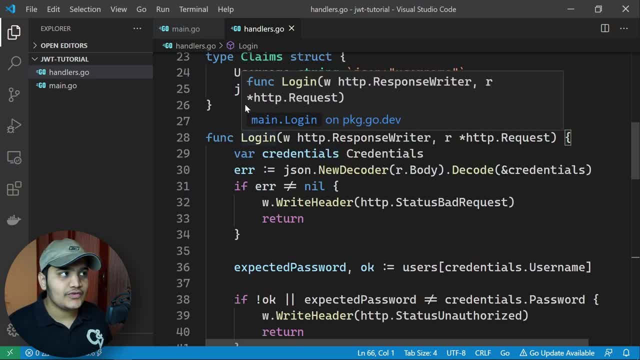 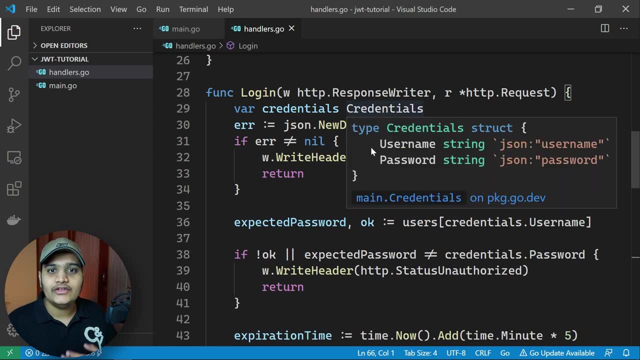 I'll just walk you through once again. Okay, So when we hit the login request over here- okay, this login request- then login handler function will be called, So it will come over here. We will be passing the username and password, So that username and password. 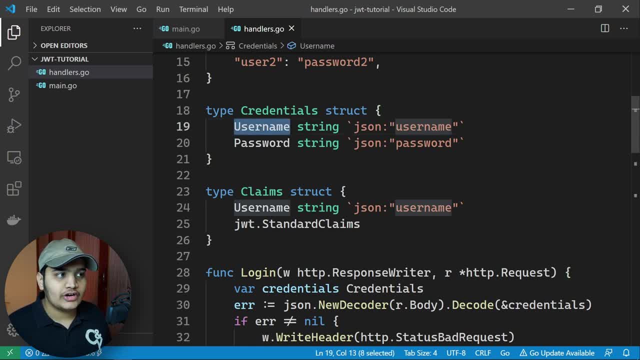 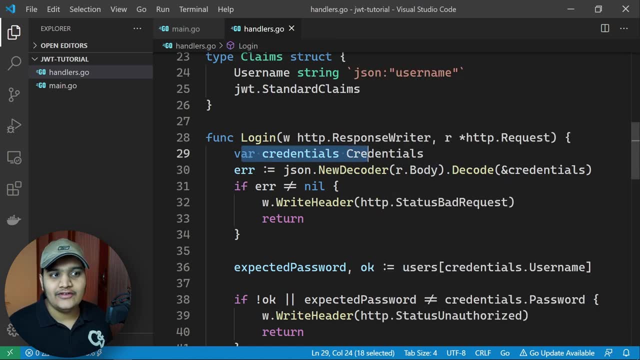 For that username and password. we have created the struct over here that will store username and password. We created the object of it and we are getting the data from the request body itself And we are decoding those information over here. If there is any error while decoding, then we will throw that. this is a bad request. 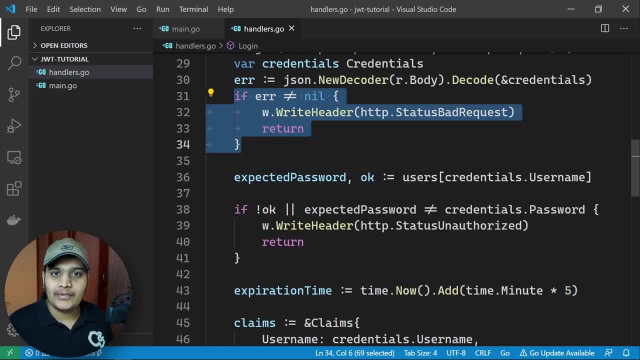 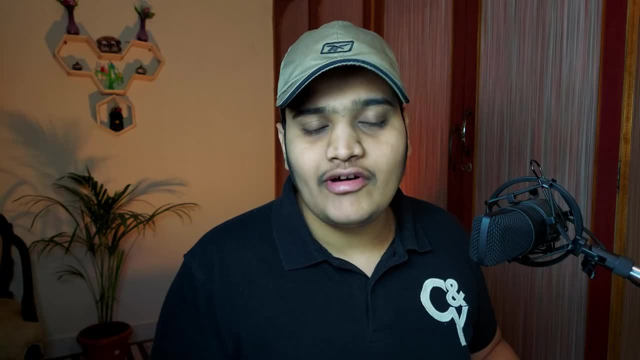 If not, then we will continue and we will check the username and password if are correct or not. We will check that username and password is the same available in our map that we've created or not In general in our production grid application. we will be checking this. 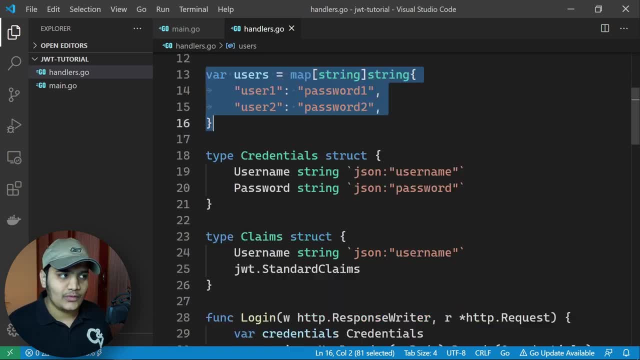 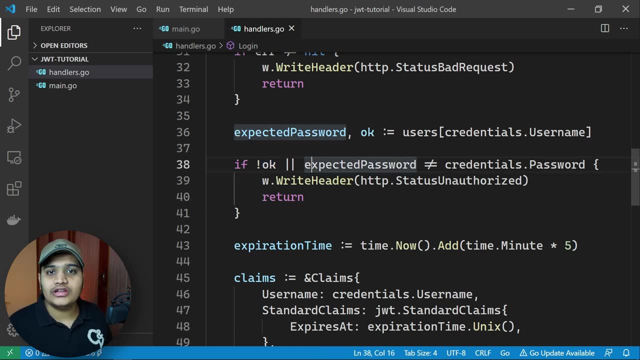 Okay, For the simplicity, we have created the map over here Once this is done. So here we will check if the data is available or not. Not okay means the data is not available in the map. So if the data is not available or the password is not matching with the password that we 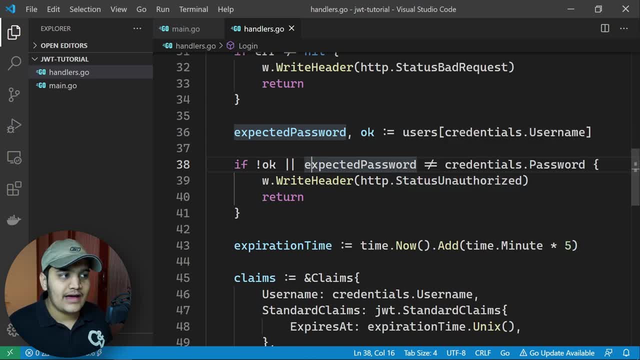 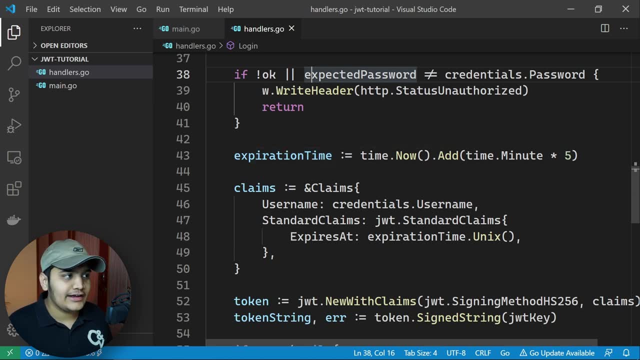 have, that means this is the unauthorized access. So we'll throw back that this is the unauthorized access. Once everything is successful, once the password is matched and we are ready to go, we are creating one expiration time for our token. That is five minutes. 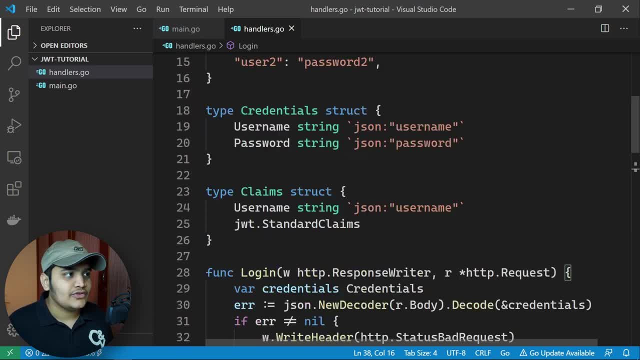 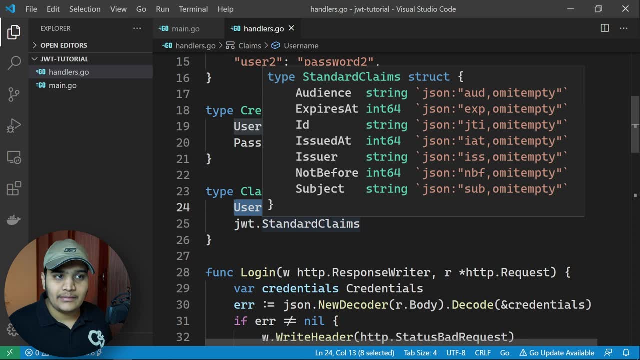 And after that we are creating the object of the claims. Inside this claim, We can see that we have created a username and then we have embedded one struct as well. So we are setting this username and inside this embedded struct we are storing the expires. 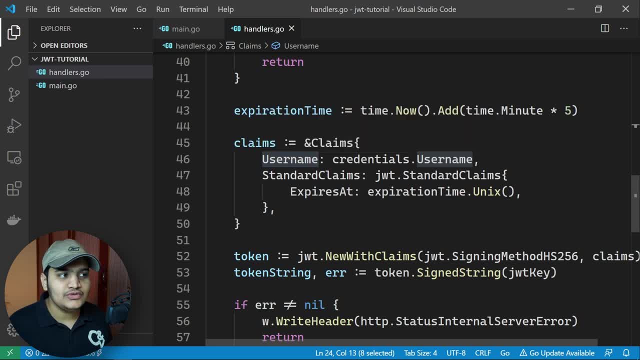 at value as well. So we are storing those information. that username equals to credentialsusername And for the standard claims, we are creating that standard claims and inside this standard claims we are using the expires at expiration timeunix. So these values that we are setting over here, 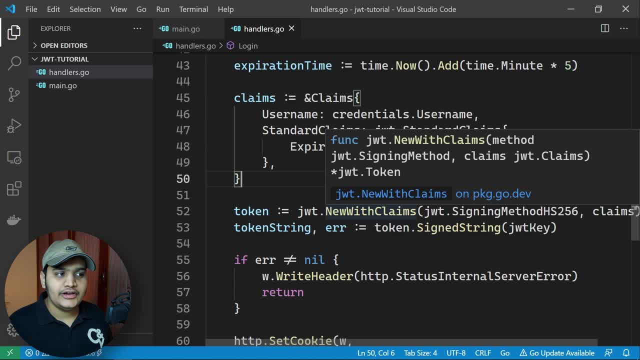 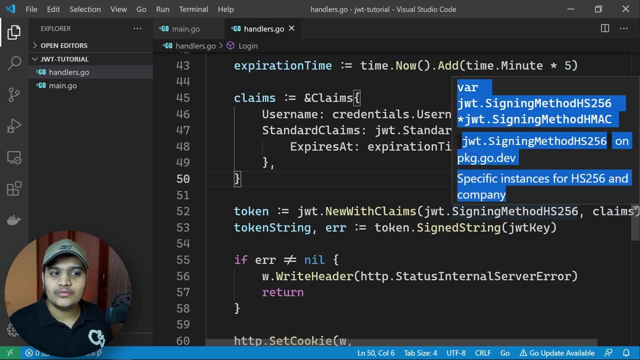 So now to create the token over here what we did, we use the JWT dot new with claims function over here And inside this function we have to pass the claims object that we have created And we have to also pass which particular algorithm that we are using to create our 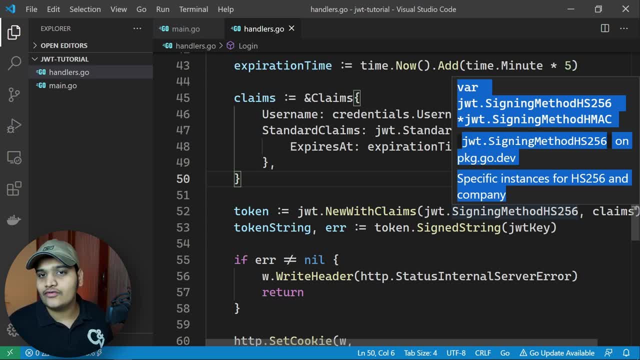 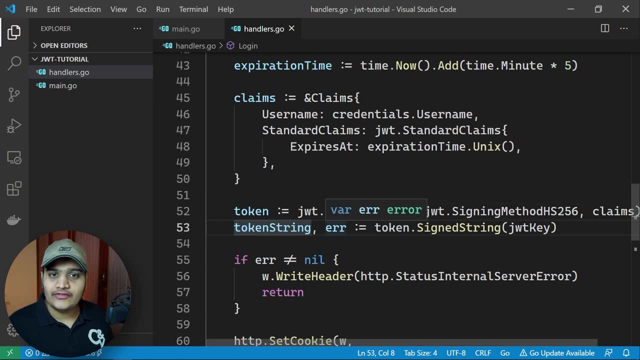 token, So we have used signing method HS256.. There are a lot of other available that you can use any of them. Once the token is created, we need to get the sign token string. So we created the variable token string and, with token dot sign string, passing the JWT. 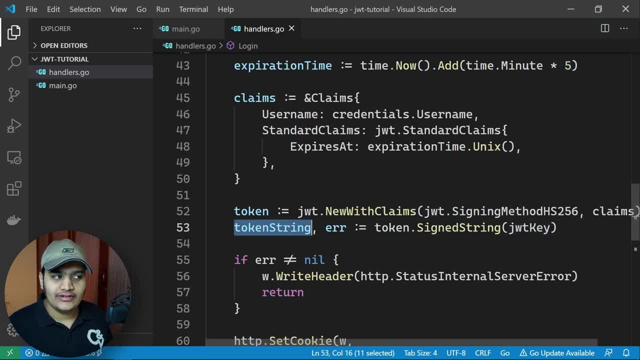 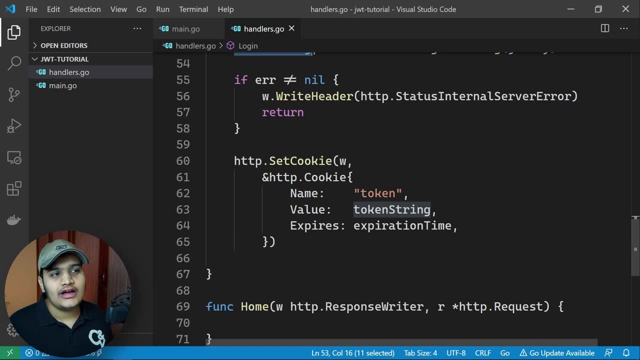 key, which is a my secret. we will be getting the token string available. We again check. if there is any error, Then throw. If there is no error, that means we are ready to go And we set those information token string, its token value and expiration time in our 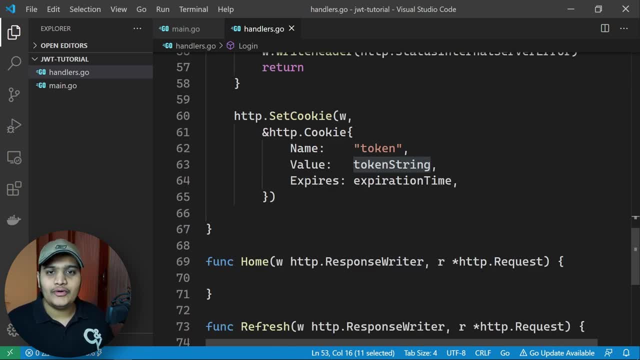 cookies. So this login method is completed. So now, in the home method, what we'll be doing is, whatever data, whatever JWT token that we are getting back, that should be exactly the same that we have sent back And if it's authenticating, if the token is valid, then we will allow the user to visit. 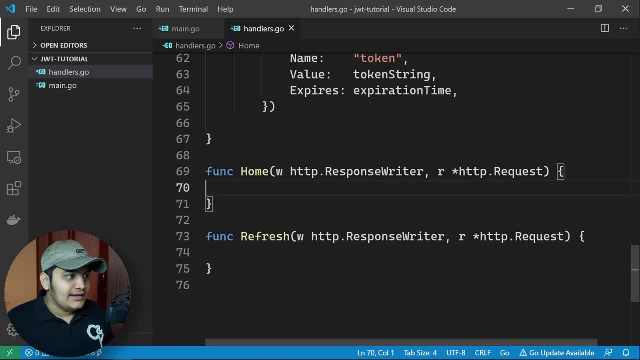 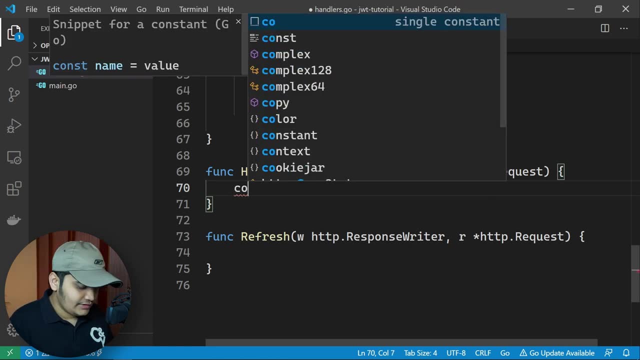 the homepage, Else we'll throw unauthorized access exception. Let's get the value from the cookie and then let's create the claims of it And let's do the authentication. So let's create the cookie variable- error variable- and let's get the data from the request. 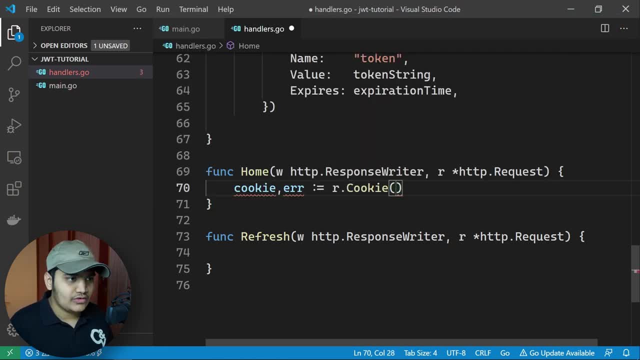 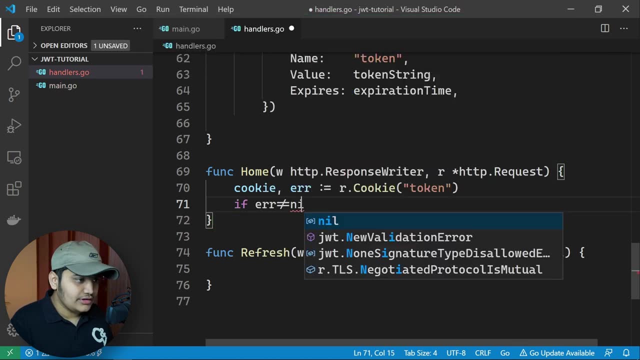 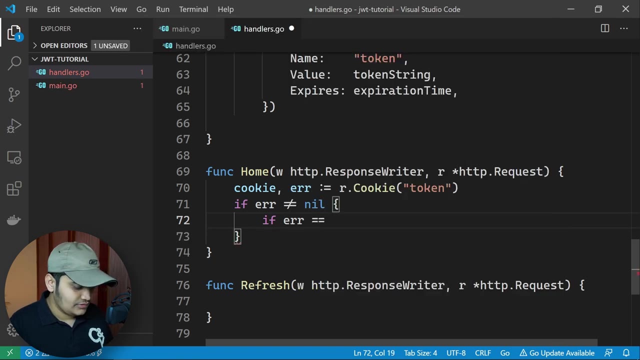 R dot cookie. And from this cookie we need to get the token cookie itself And we'll check. if error not equals to nil, Okay, Here we will check. if that error equals to equals to error, no cookie, So, And here we will check if there is no cookie. 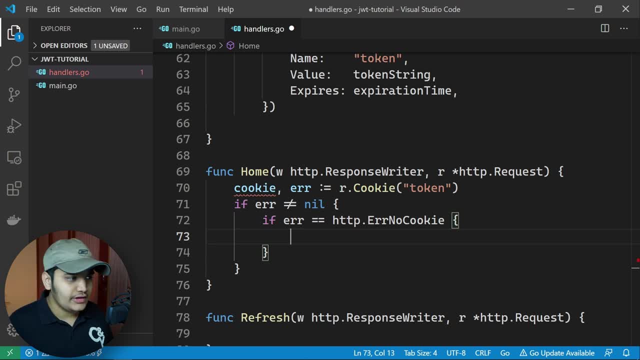 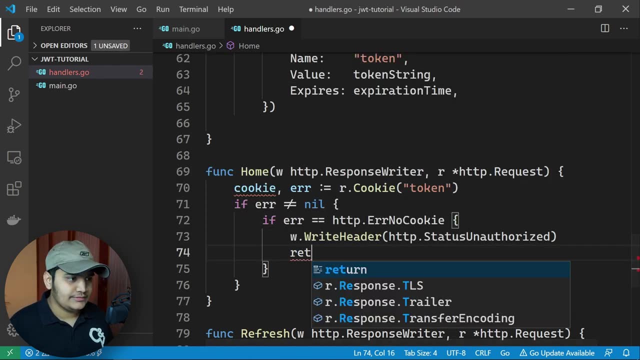 That means that's an unauthorized access. We need a cookie with the token. Okay. So we'll say WD dot write header unauthorized and we will do return that is of not this type. Then we will say WD dot write header. That is bad request. 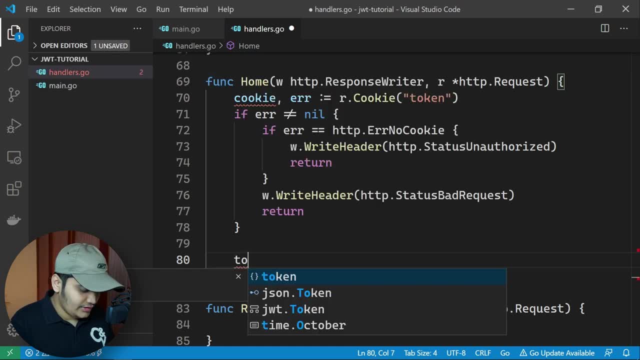 This is simple. So now let's get the value of a token and set over here. Token str equals to cookie Cookie dot value. Okay, So we got the token string from the cookies. Now let's create the claims object over here. 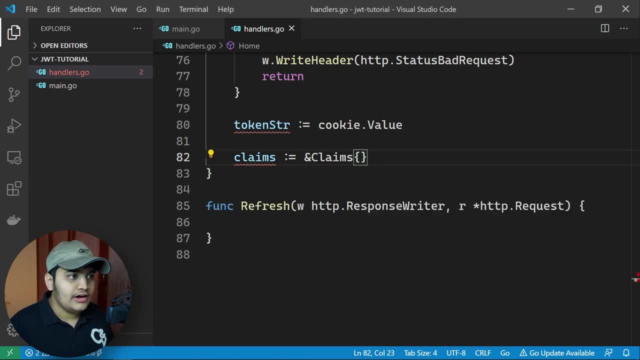 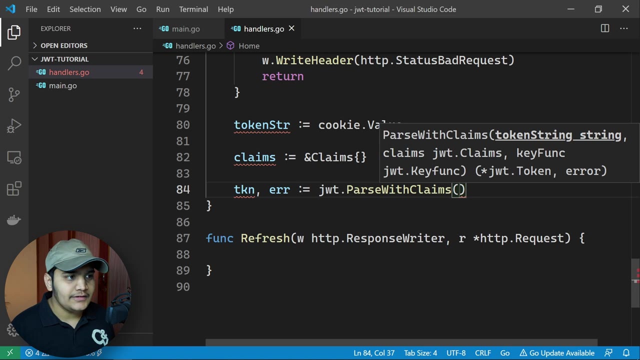 Claims equals to reference of claims, And here we have to parse the claims back using the token string and JWT key. So let's create the token error JWT dot- parseWithClaims over here Inside this particular method, parseWithClaims, we have to parse the token string claims and 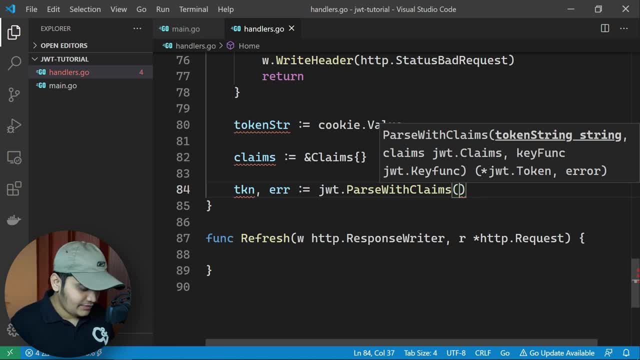 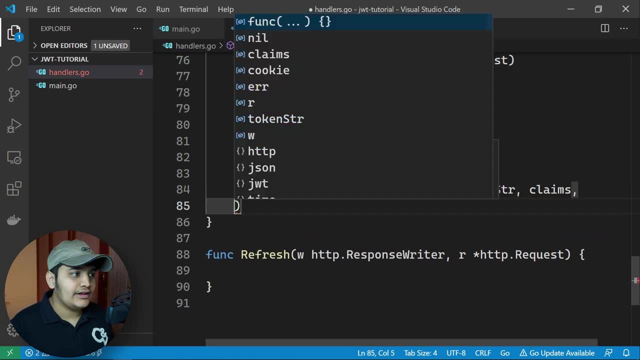 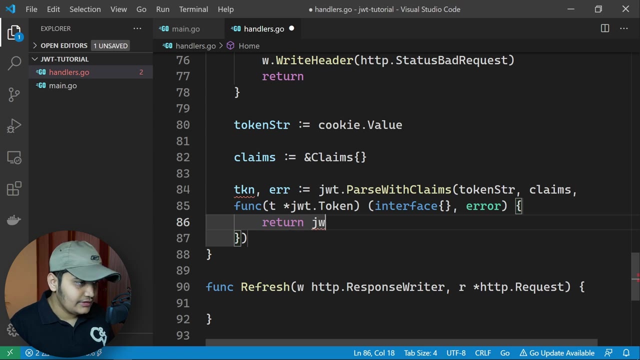 the key function over here. So let's parse this information over here. We'll pass token str, then we'll pass claims over here and then we'll pass the function over here. That function should return the JWT key and nil. That is the error over here. 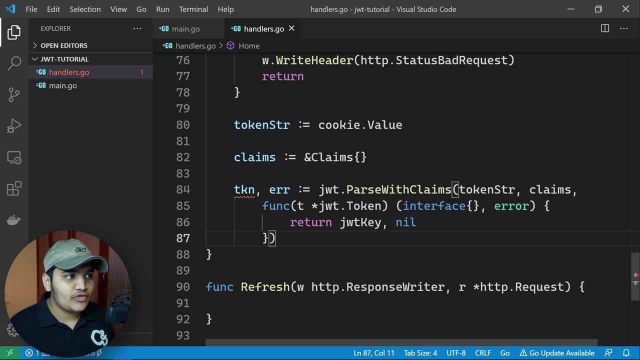 So this particular parseWithClaims function will return the claims over here. Okay, This particular things claims object over here with using the token string. Okay, The token string claims particular object and the JWT key information. Now, here we'll check if error not equals to nil. 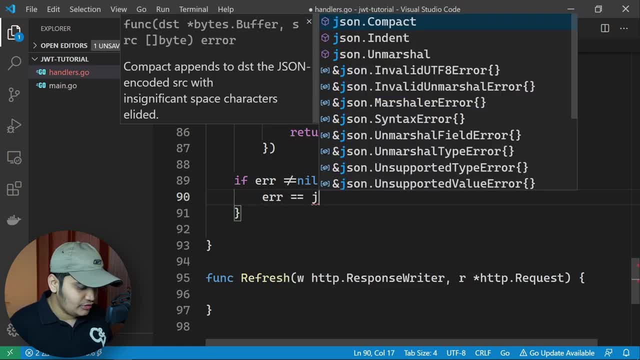 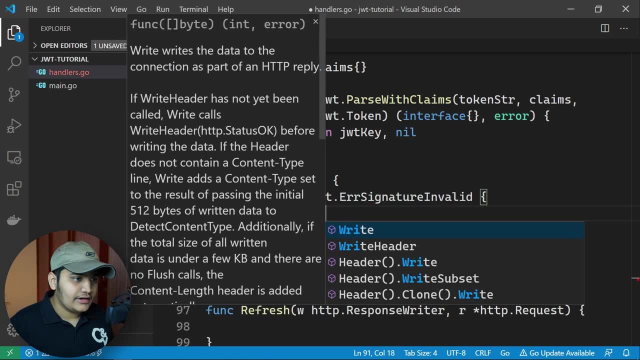 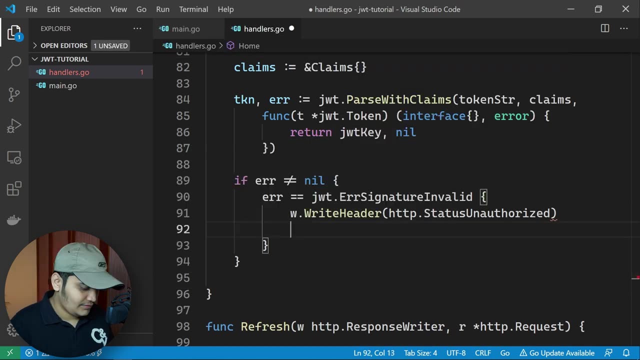 And then this particular error equals to, equals to of JWT dot. this error dot signature invalid. If this is this particular error, then we'll write wd dot, write header: unauthorized signature, unauthorized access, and then we'll return: Okay, Okay, Okay. 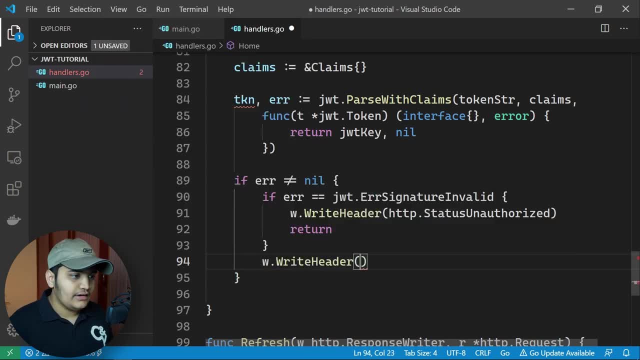 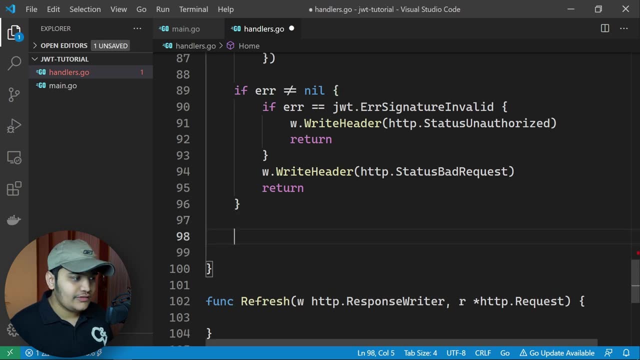 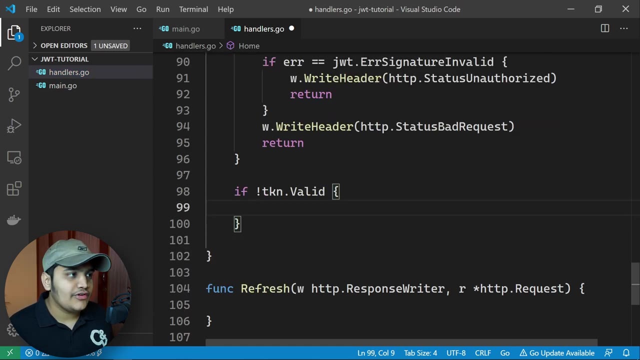 And then tkn- dot unauthorized access, We'll return. Otherwise we'll say w dot write header, bad request return. If there is no error then we'll check if token that we have got that is valid or not. The token that we got over here that is not valid tkn, then we'll say w dot write header. 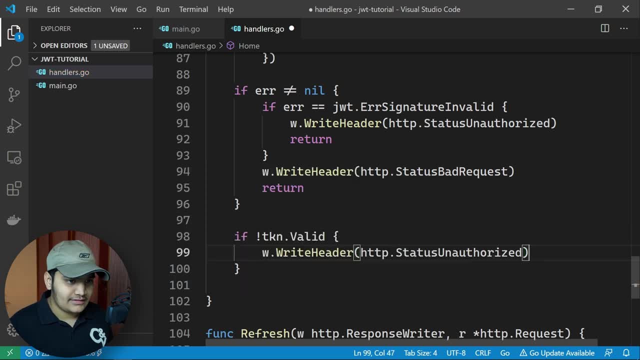 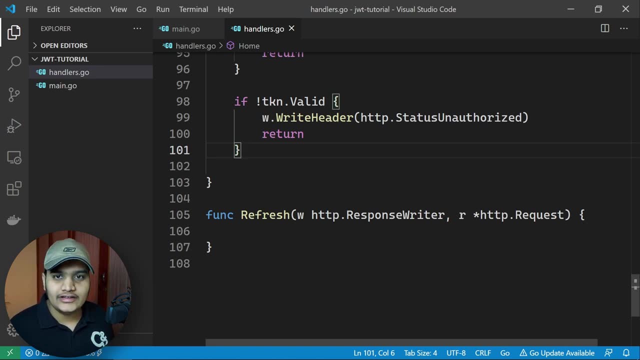 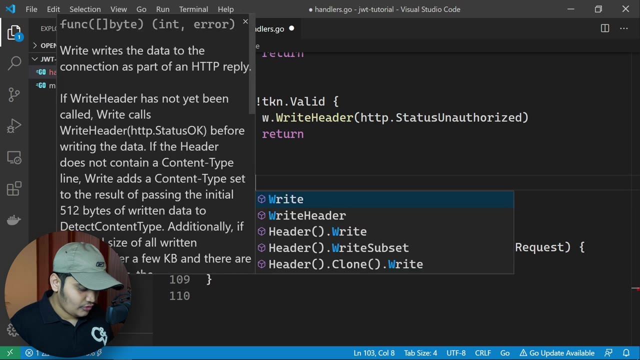 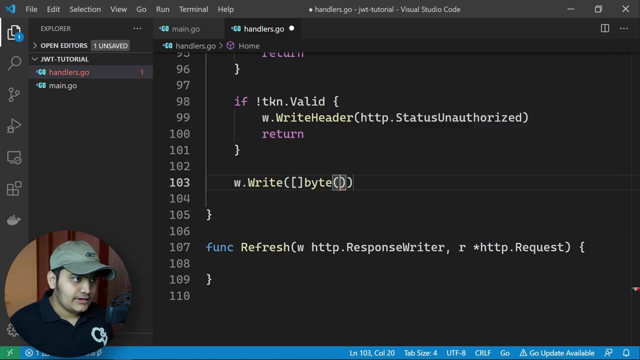 unauthorized access and we'll return. Now. that means here, if we checked everything, that means our token is valid. now, if the token is valid, then we will pass the information and we will allow user to enter our home page. so we'll just say w dot write, and we will write with the byte array and here we'll say fmt, dot, sprintf. here we say: 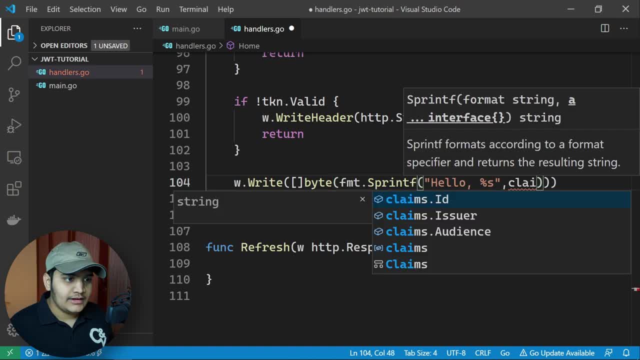 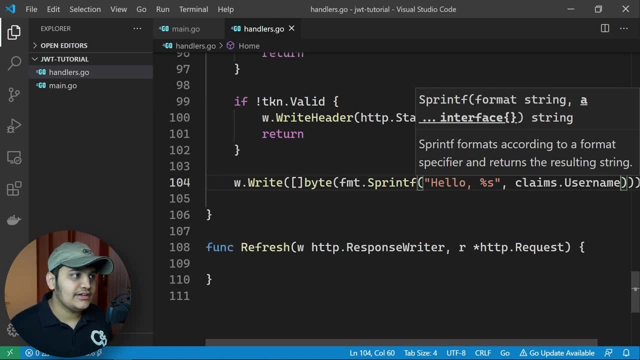 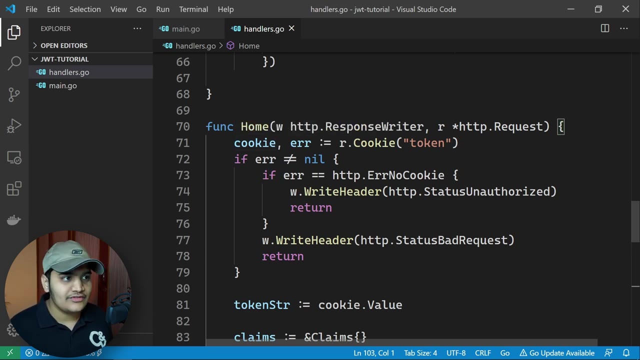 hello user, and here we'll pass claims dot username. so we are writing back that welcome, whatever the username it is. so once everything is authenticated. so what we did over here? it's very simple: over here we got the cookie from the request itself, from the token name that we are setting over here. 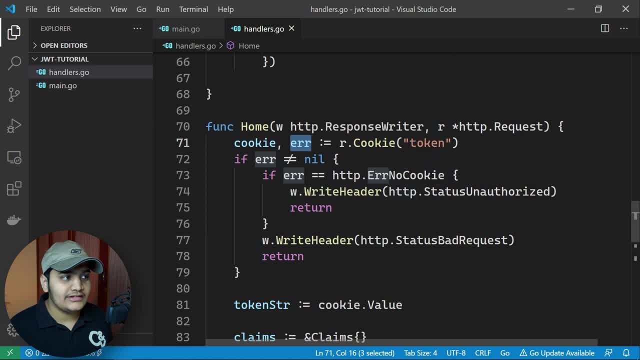 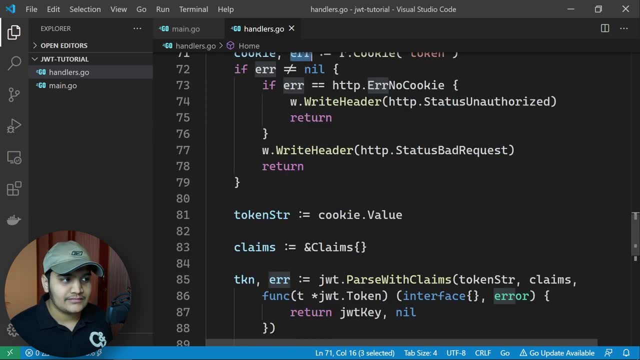 once we got the cookie- and we are also checking this particular error- that this error is of type error- no cookie- then that is status unauthorized. if it's not this type, then we'll say bad request. if it's valid, then we are getting the token string from the cookie dot value. 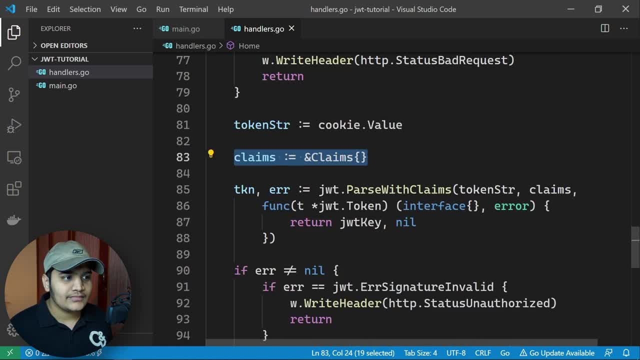 and we are creating the reference of the claims over here, claim struct and with the jwt dot parse with claims function over here. we are passing token string, claims, object and the function over here. that is returning the interface. and we are passing the dwt key over here. this will return the. 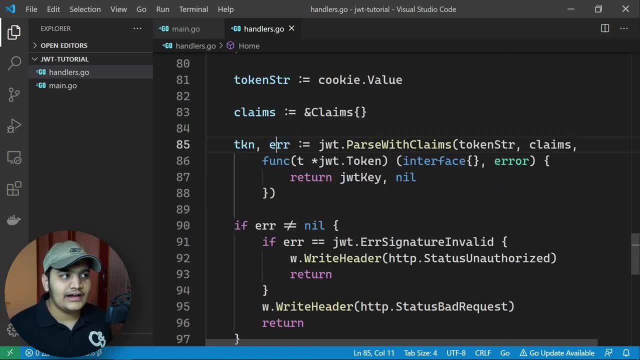 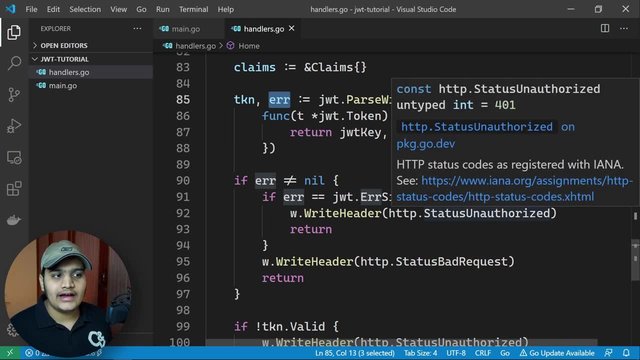 token over here- and we are checking the again error over here- that if that particular error is not nil and that particular error is of type error signature invalid, then we are throwing the error that it is an unauthorized request and if it's not of this type we are saying that it's a. 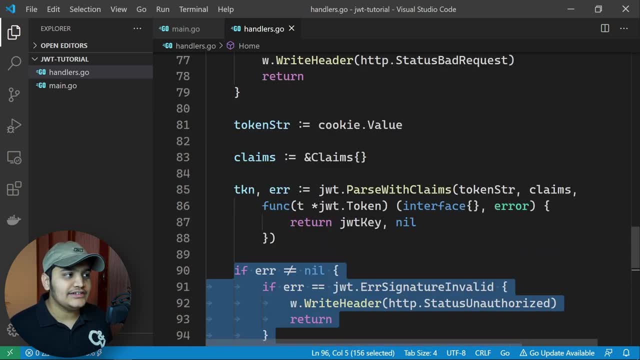 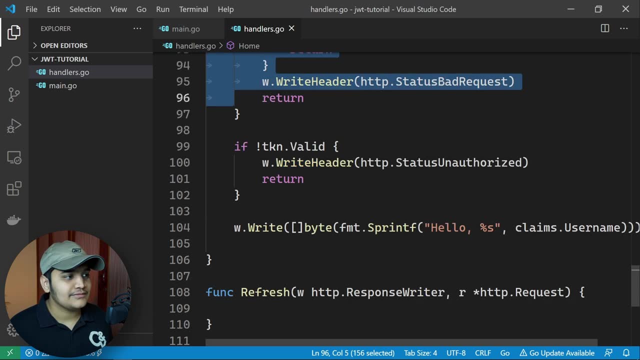 bad request. if there is no error. that means after that we are checking that if this particular token is valid or not. if this particular token is not valid, then we are again saying that is unauthorized request. after this: at the last token is valid. so once the token is valid, 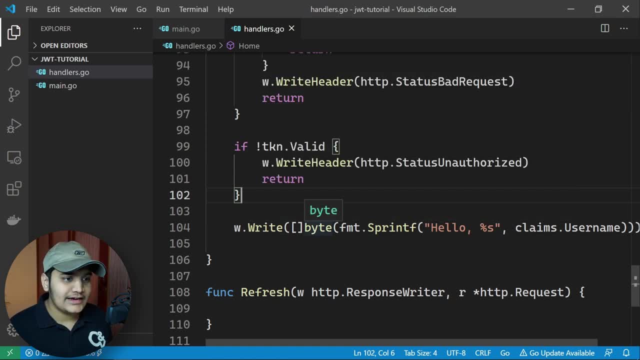 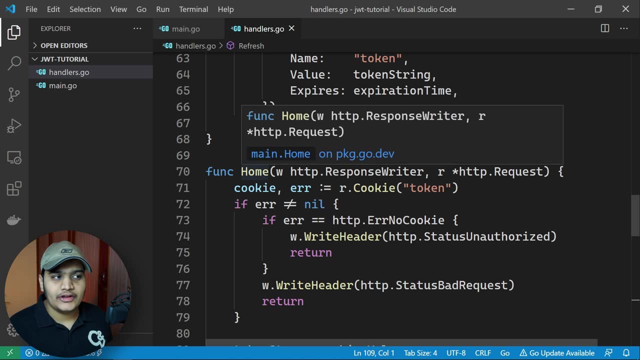 we are passing the data back to our client in the request and saying hello, whatever the user name it is. so let's run this application and check before implementing the refresh. when we use this home particular function over here, when we call this home api without passing the token information, we are not allowed, and if we pass the token information we should. 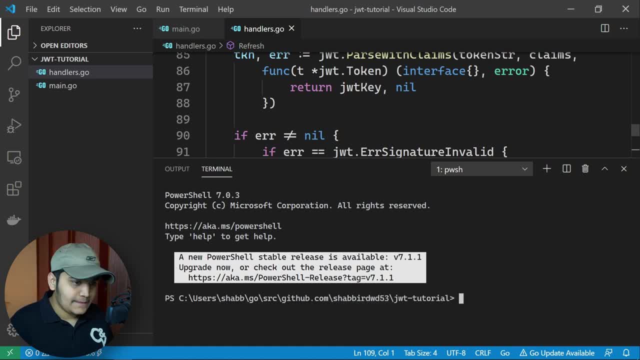 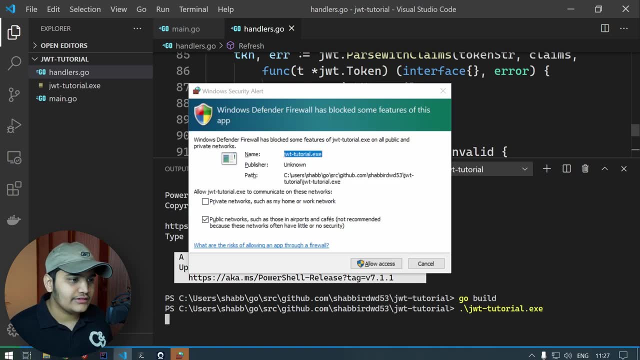 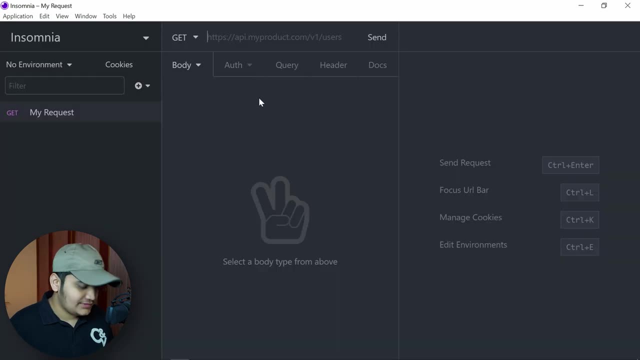 be allowed. let's run this. we'll say go build and we'll say jwt- tutorialexe. we'll run this. now. let's go to insomnia. you can use anything, okay, now let's create the new request and request. here we'll say: http: localhost colon 8080 is our port number. slash home is the. 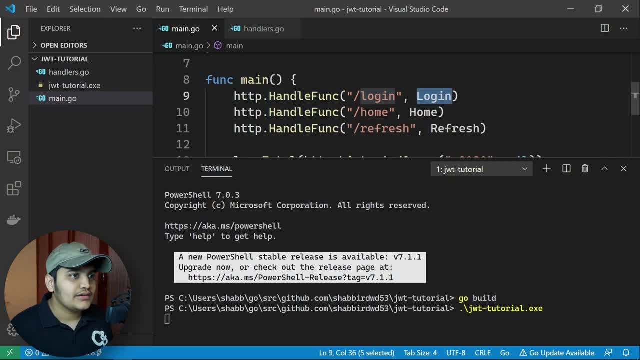 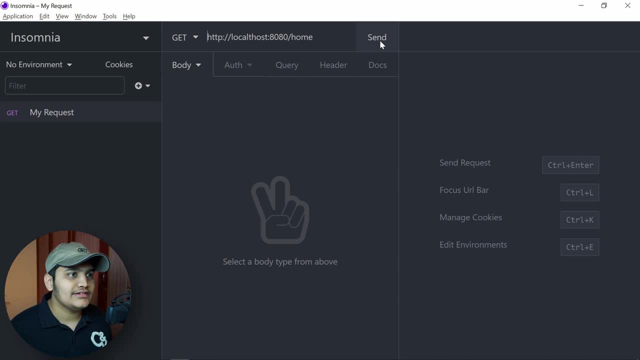 api. right, we'll go to main home. is our api? okay? so we'll call this. and our port is 8080, so let's call this. okay, let's do send spelling mistake again. we'll do hit send again, okay, and here you can see that we are getting unauthorized access over here, this particular request. 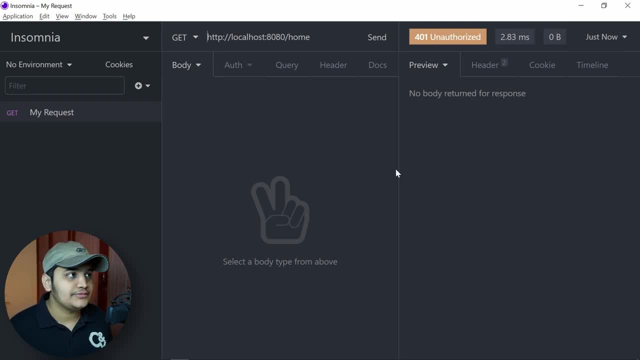 home we are not able to authorize because we don't have token information. so now let's get the token information, let's get the token, and then we will hit home over here. so to get the token we have to log in first. so we'll do login inside this body. we have to pass. 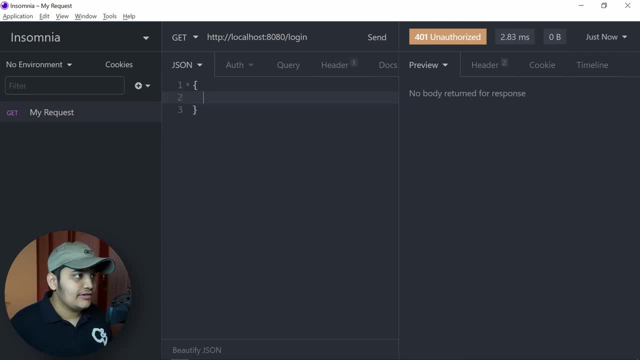 the json data and we have to pass username, user name, colon, user. one password is password one over here. That was the password that we have stored over here. Let's check that again. This is the one. So let's change to post request and let's give the wrong password. 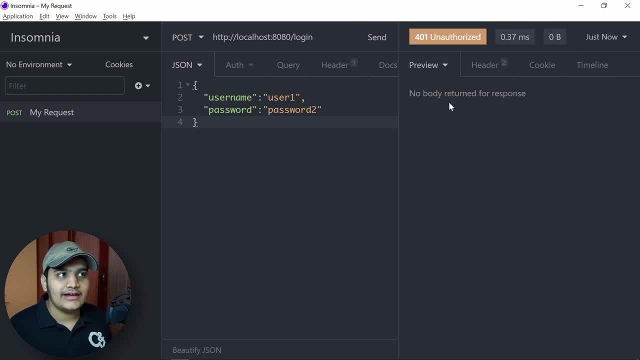 over here first and let's check what's happening over here. Okay, you can see that we are getting the unauthorized access, So that means we are not authenticating the data over here. The data is not correct, So let's pass the correct data and check what's happening You. 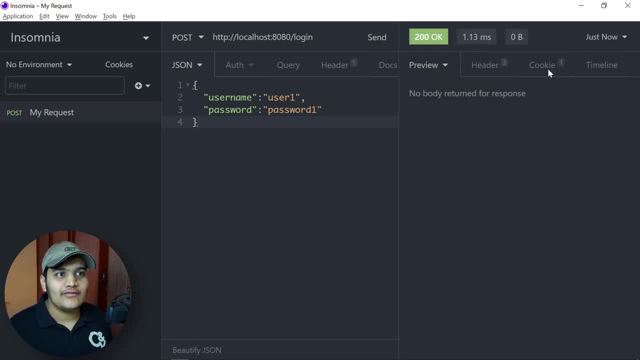 can see that we are getting 200 okay over here. And one more thing is we got the cookie as well. you can see that the cookie name that is token over here and we got the value also. So if we, if you copy paste this particular value over here and if you check in the JWT- 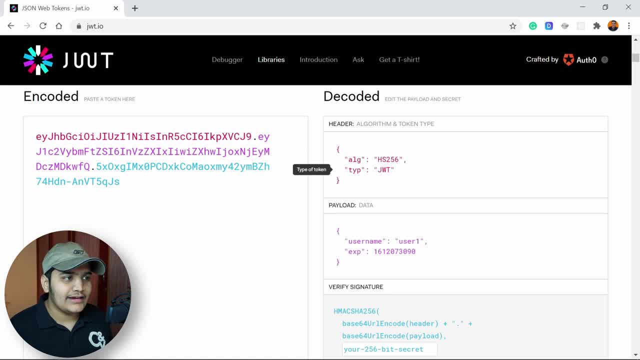 over here. you can see that you are getting the particular header and payload data as well. Okay, the header is hs 256.. This is the algorithm that we have used, And in the payload data you can see that my username is user one that we set over here. So we have. 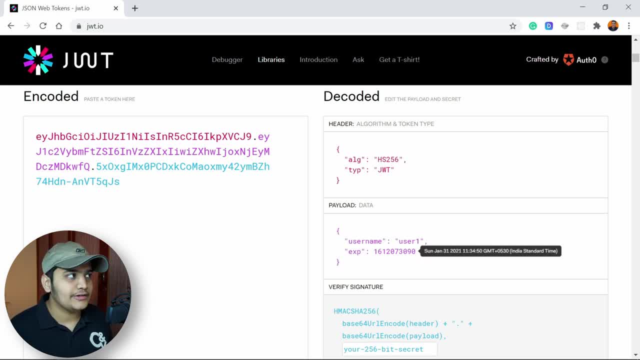 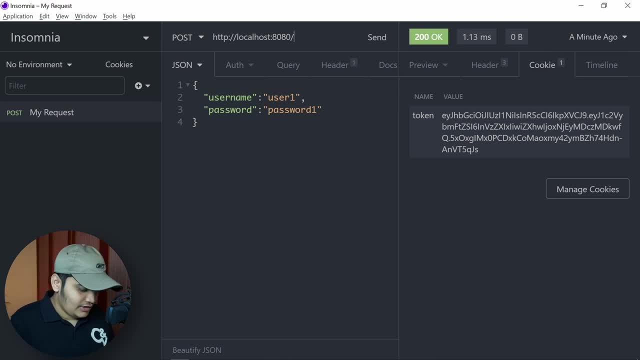 here and the expiration time is this particular thing. you can check the data as well over here. So we are getting the token over here Now. after this, after we get the token over here, if we go to the homepage over here, let's change to get request and if I send, 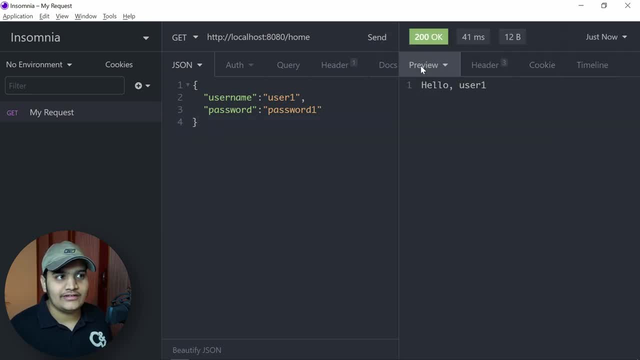 Okay, then you can see that my request is successful And if I see I'm getting Hello user one, okay, so we are able to authenticate and authorize our request using the JWT token over here. So till this particular cookie is available, okay, if I go to manage cookie. 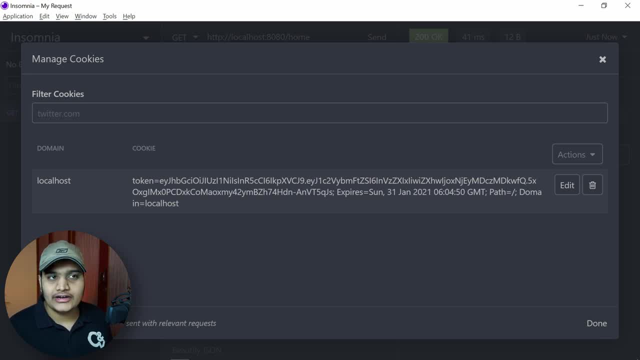 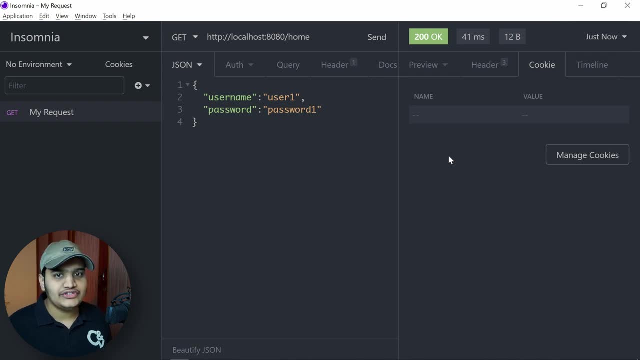 till the time. you can see the expiration time is there. till this particular time this cookie will be available And till that we'll be able to authenticate the token. So this is how you will be doing the authentication and authorization, using the JWT we created. 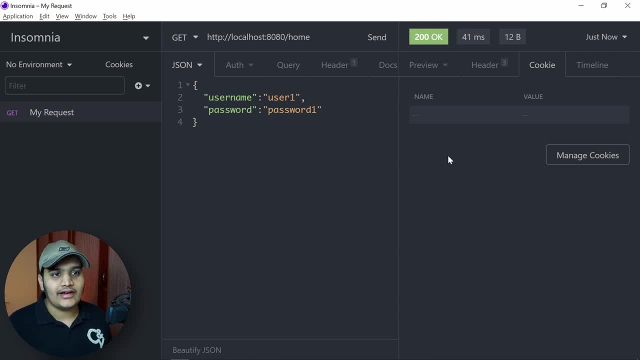 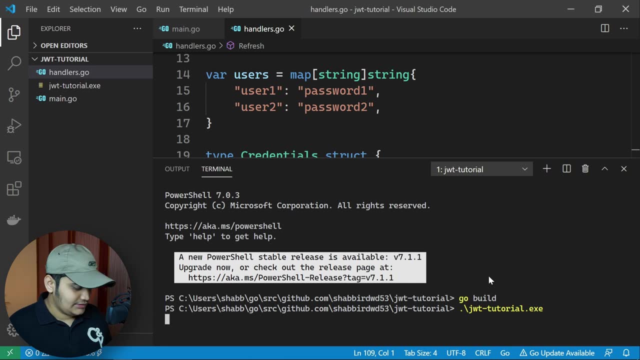 the home request and we created the sign in request, login request. we are creating the token and we are calling the homepage as well. Now let's go ahead and do the refresh token as well. Stop the server Now. let's go to the refresh method over here Now, inside this: 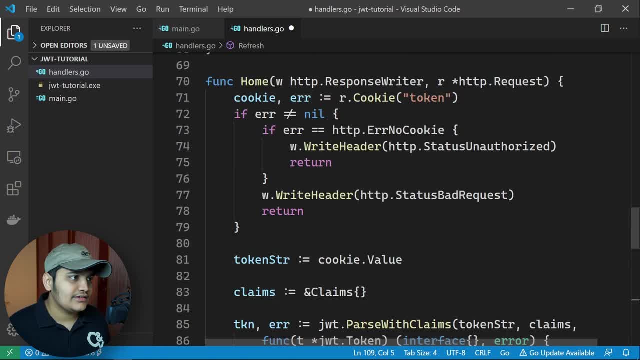 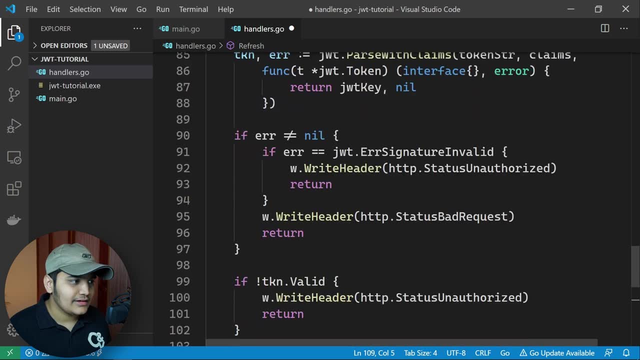 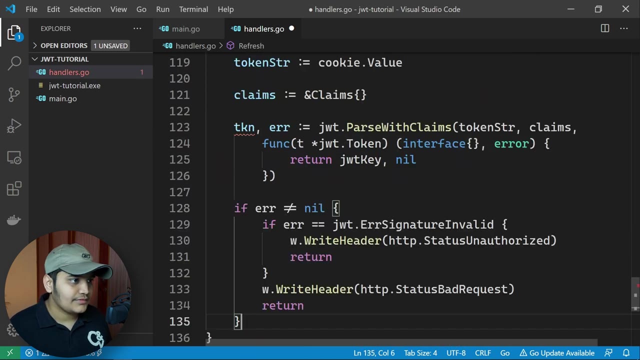 refresh token. also, most of the things for the home will be same, because we will be taking the token, we will be authenticating the token. all those information will be same till here. Okay, so we'll copy paste all this information. So here also, we are getting the token, we are 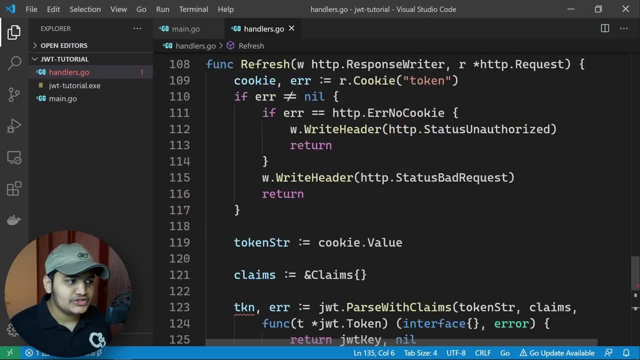 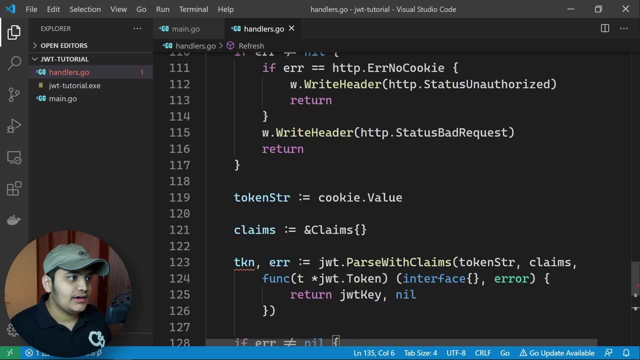 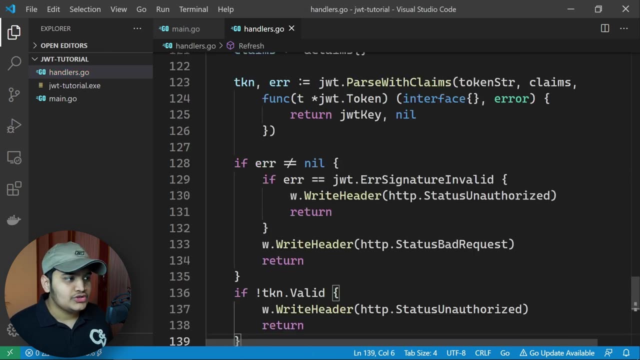 taking the token information over here. we did all the validations over here. we created, we got the token string, we created the claims out of it. We again check all those information and we will also check the token is valid or not over here. So till here we did similar. 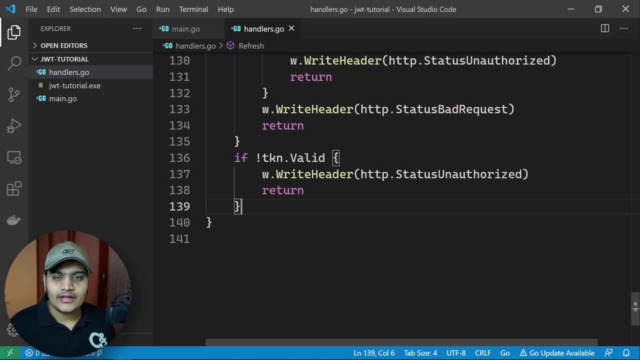 to the home method. over here we get the token from the particular request and we did all the validations over here. So once everything is valid, we have to check the time interval now. okay, so we'll check if it's about to expire that particular token at that time. 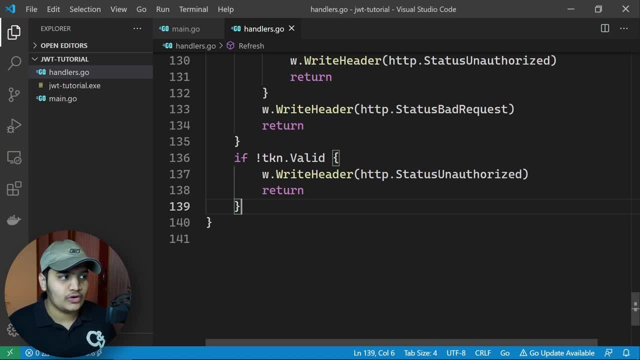 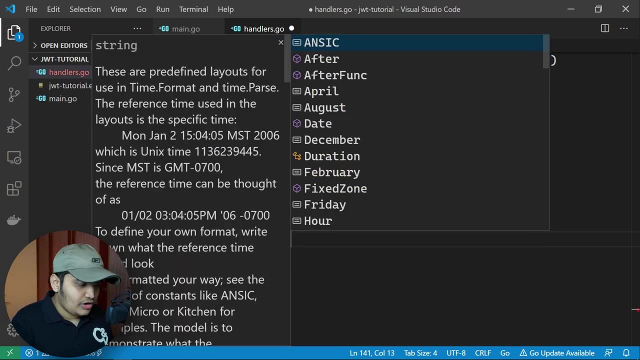 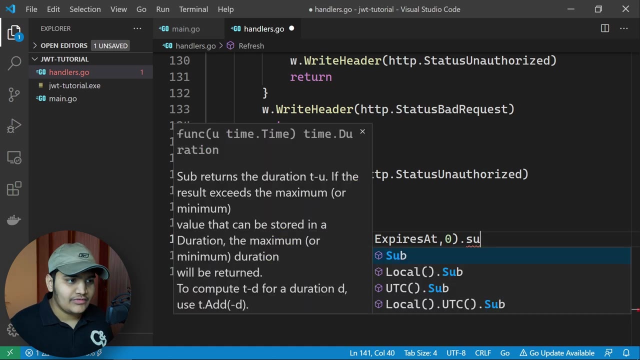 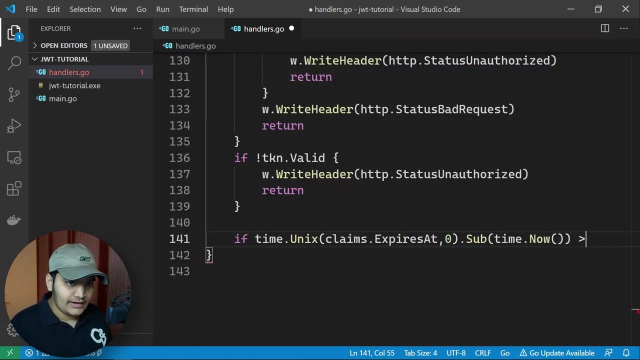 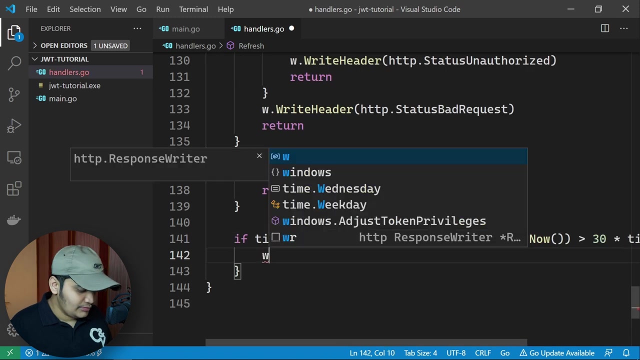 we will create a new token, will create a new refresh token and we will pass a token over here. So let's do that thing over here. So we'll do. if time dot unix claims that expired at comma zero, and we'll subtract the current time from it. subtract time dot now and if this is greater than 30, into time dot seconds. 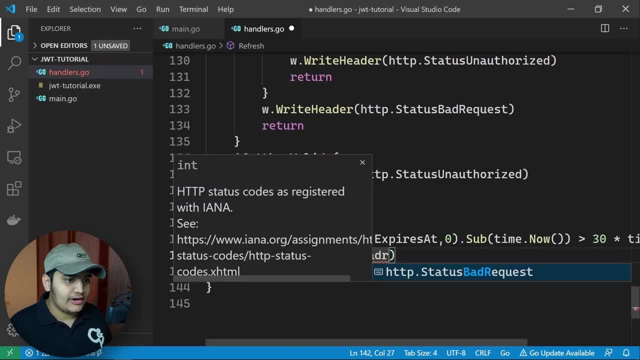 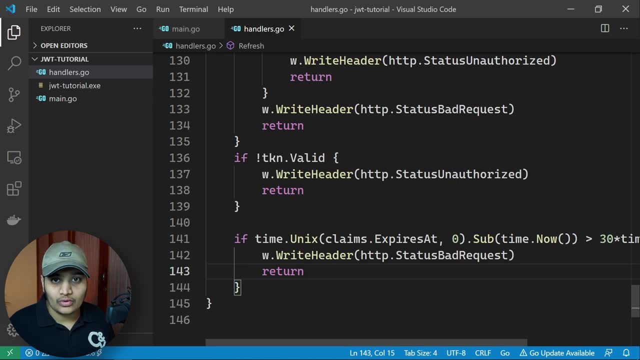 W dot write header by request. So this is a simple check that we added over here that if we have provided the five minute token interval expiration time, then if the time interval is around 30 seconds remaining, at that time we can refresh the token. 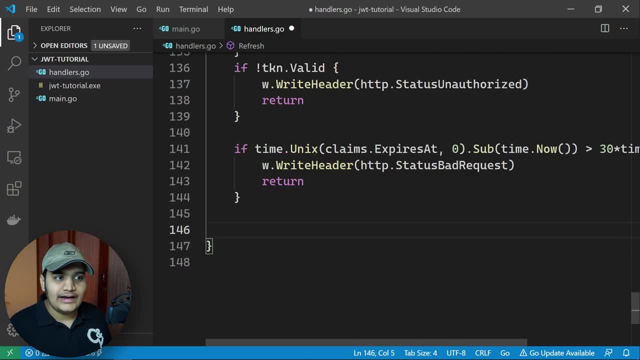 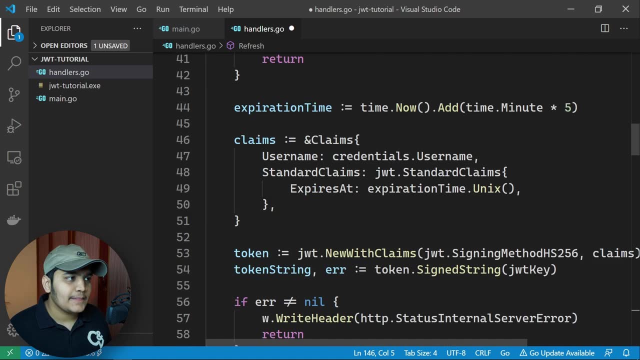 You cannot refresh token every time, So this is the check for it. After that, we have to create a new token. So to create a new token, we will go to this particular thing over here. Expiration time. So we need expiration time claims information. 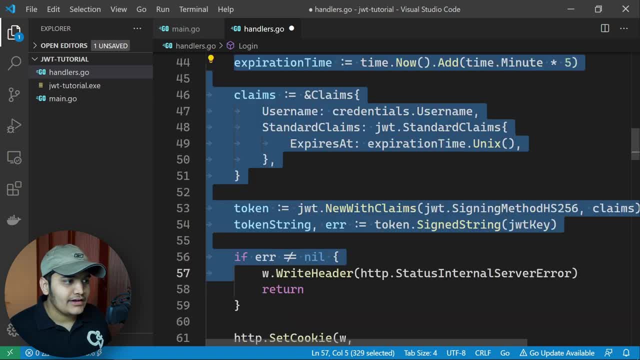 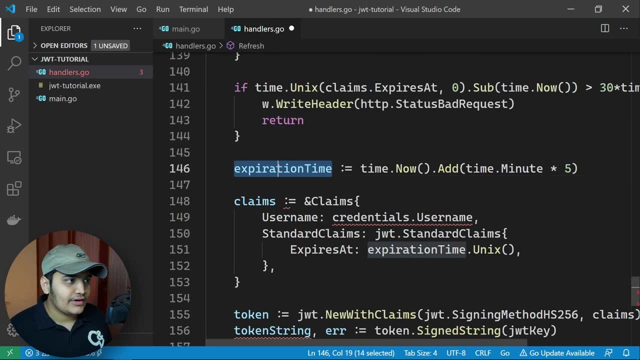 This is the token And we again have to check this error is all things we have to do again, So we will do all those things back again. So expiration time we got. okay, we don't need this information because we have already have the claims object. 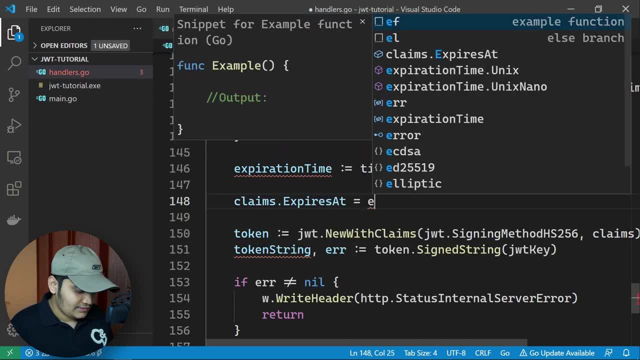 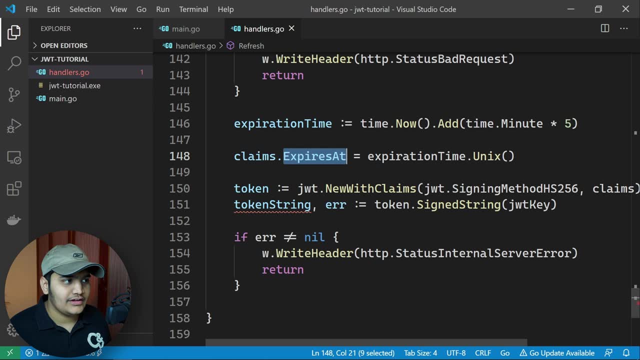 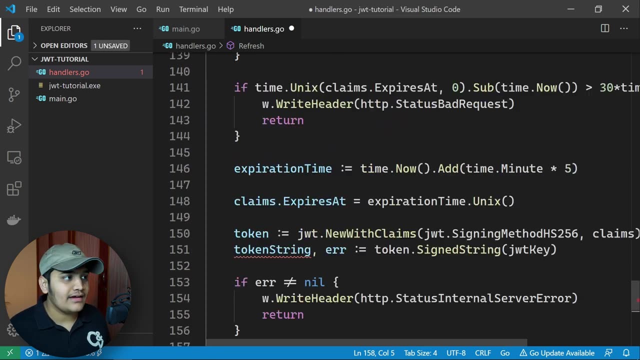 So we'll just do claims. dot expires at expiration time. dot- unix. So we set the expiration time again over here. we created the token with the same method and we got the token string. We validated the token string and once this is done, we can set the cookie back again. 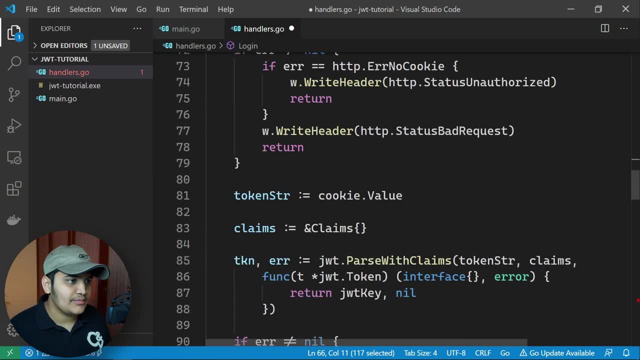 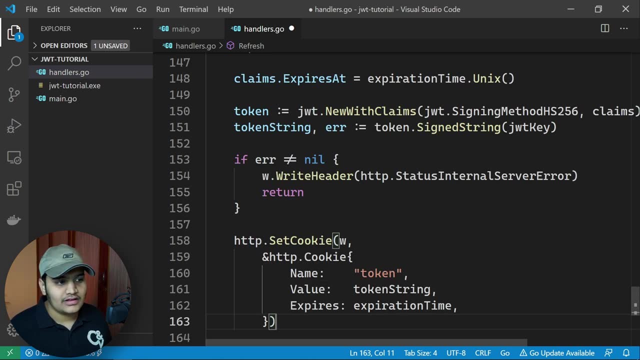 So let's set this cookie will copy from here, okay, and we'll paste the cookies over here Now for now, for the simplicity is you can understand. so I'm just changing the name over here So you can directly identify that new cookies created for now. 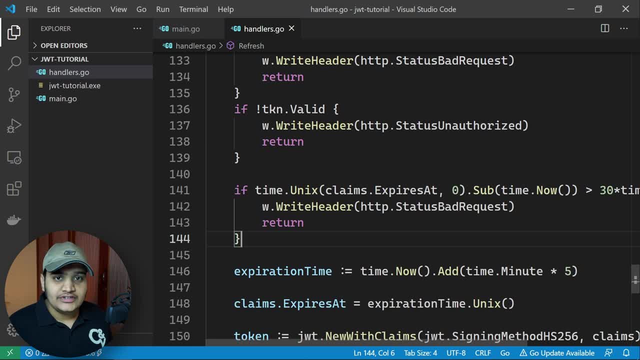 Okay, Otherwise you'll be using the same one. So, for the simplicity also, I'll just remove this condition over here For the 30 seconds. that at the last 30 seconds only you can create the refresh token. I will just remove for now. 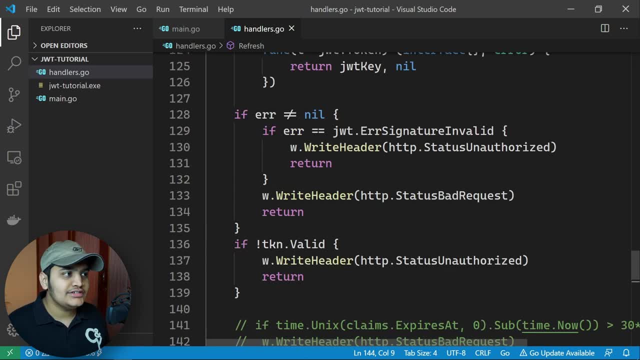 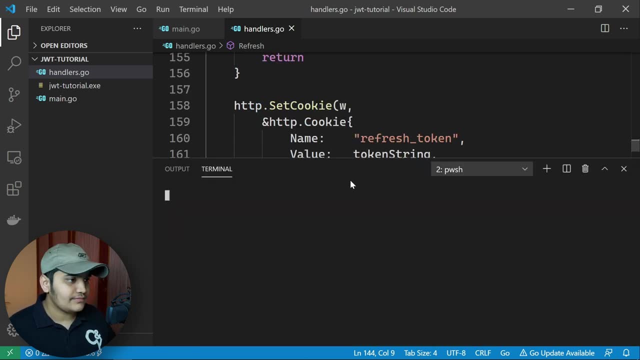 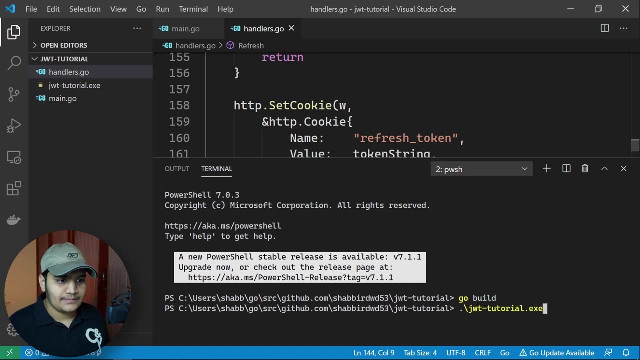 So we can check instantaneously. okay, we don't have to wait for it. So this is just a refreshed method that we have created to refresh the token. Now let's run it again And let's see what's happening. will do go build and JWT tutorial. 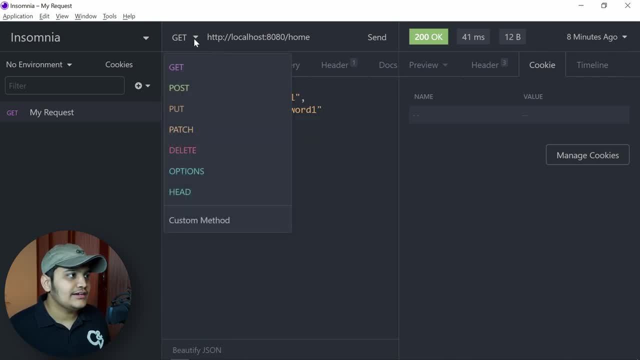 So this is running. Let's go to insomnia. Let's do the post request To the login over here. hit on send and you can see that one cookies created. If you go to manage cookies also, there is one cookie available with the token name. 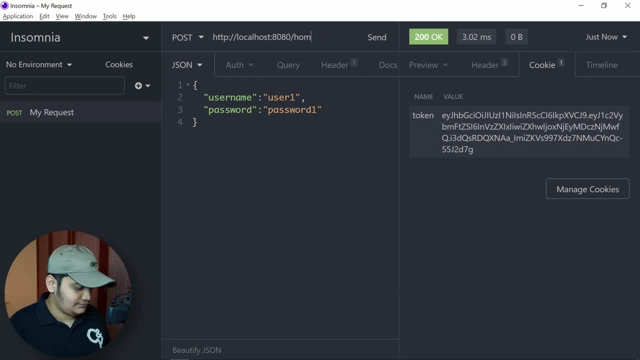 After that, if you go to the home page, we are allowed to access this particular page over here. Now suppose after the four, four and a half minutes of time, you are thinking that your cookies will be expired, you will be creating the other refresh request to refresh your. 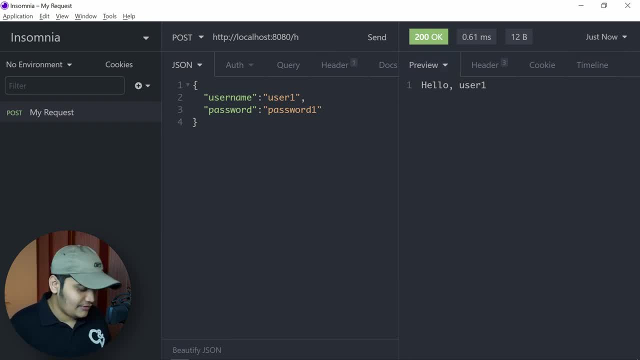 token itself. So let's do that Now. itself refresh token. And yeah, you can see that once we hit send over here, you can see that new cookies created with the refresh token over here. So my old cookie was validated and then, accordingly, new cookie was created. 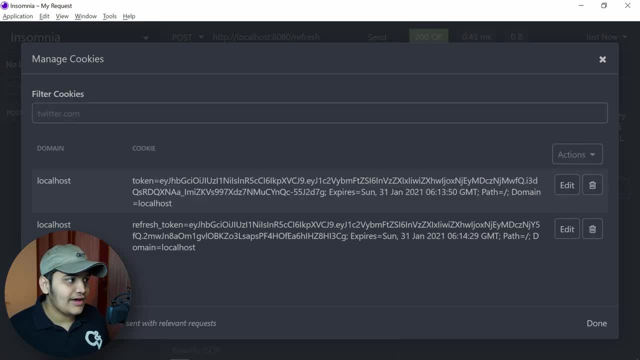 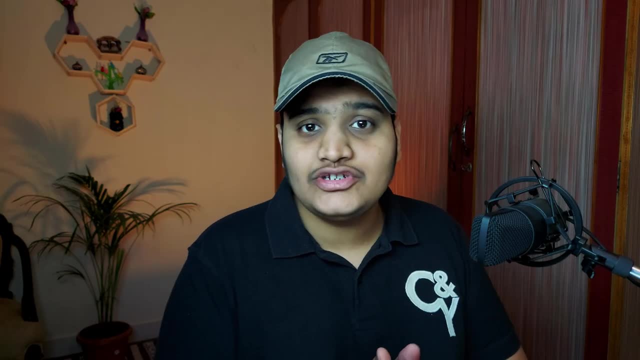 So if you go to the manage cookies over here, you can see that we are having two cookies over here. So this way you can call the refresh token as well when there is a expiration time nearby. and all this management has to be done from the client side, because client is responsible. 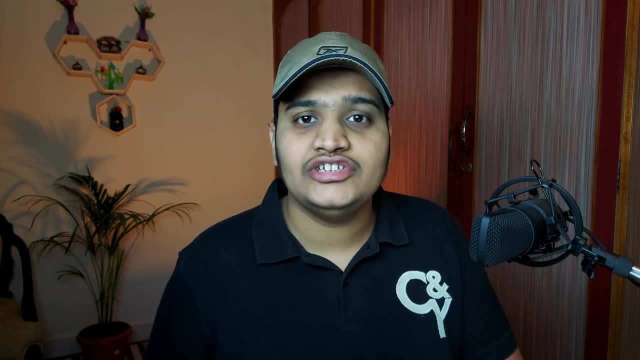 So let's do that. So let's do that. Okay, So that's how you can send the JWT token for every request for authorization and authentication When you're working with the microservice. that's a point that we have to take in mind. 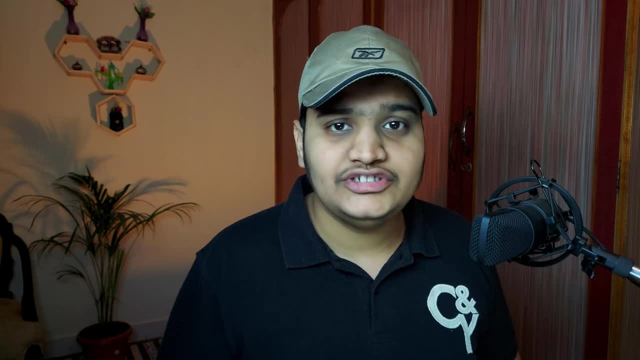 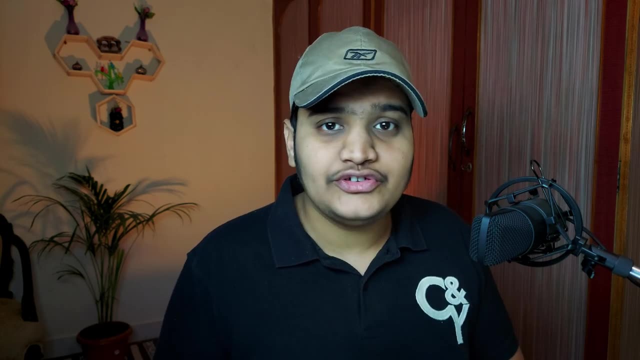 So that's all in this video: how to create the JWT token and how to use JWT token for authentication and authorization of your Go APIs, and how you can create the refresh token also to refresh your tokens at every interval. So I hope you have liked this video. 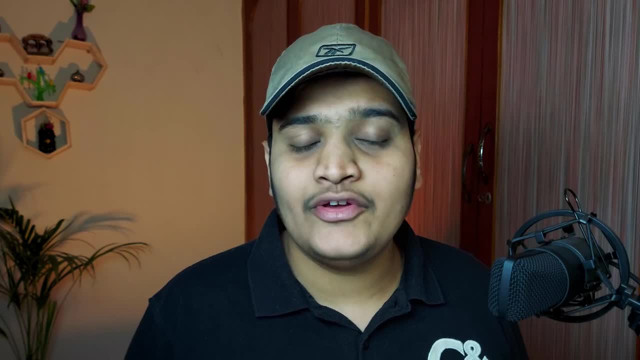 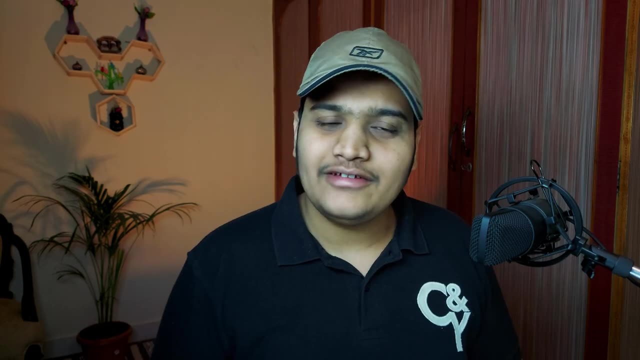 And if you like this video, give us a thumbs up and subscribe to my channel for the upcoming videos. You can also follow me on Twitter and Instagram with the same handle, dailycodebuffer, and we can chit chat over there as well. So till then, happy coding, bye, bye.